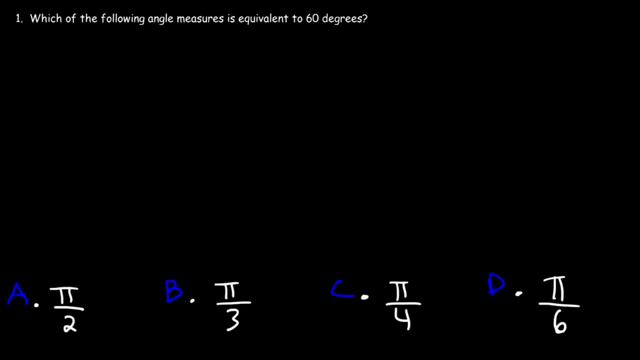 In this video I'm going to focus on solving basic trigonometry problems. Now, what I recommend that you do is pause the video and work out the problem first. Once you select your answer, unpause it to see the solution and how to arrive. 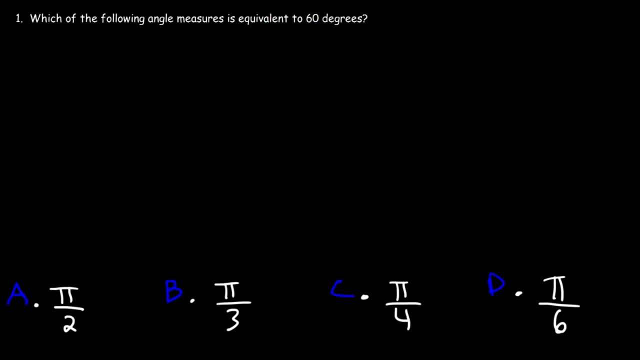 there as well. So let's start with this problem. Which of the following angle measures is equivalent to 60 degrees? So basically, what we need to do is convert degrees to radians. So how can we do that? The best way is to multiply by pi. 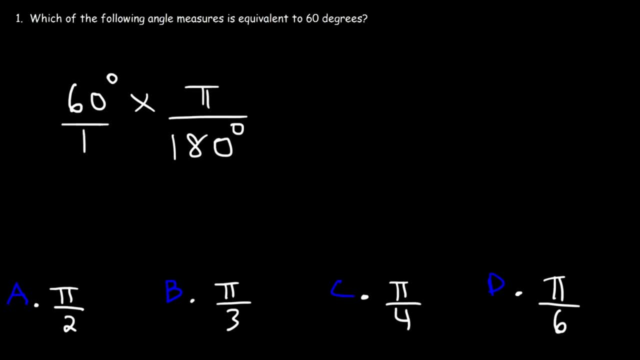 divided by 180.. You want to set it up in such a way that the degree symbol cancels, And so this becomes 60 pi over 180.. Now how do we simplify this? For one thing, we can cancel a zero. 60 over 180 is the same as 6 over 18.. And 18 is. 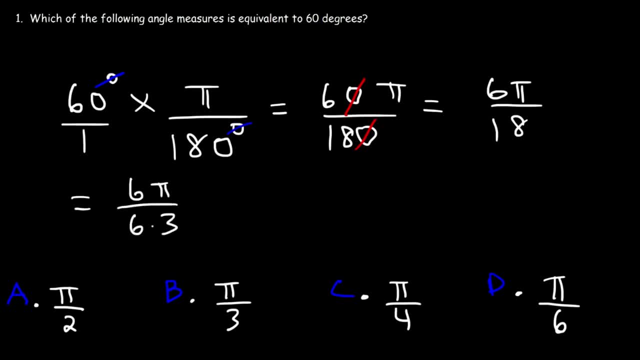 6 times 3.. So now we could cancel a 6.. And so 60 degrees is equivalent to pi over 3.. And so that's a simple technique that you can use to convert degrees to radians. So therefore, B is the right answer, Number 2. Which of the following: 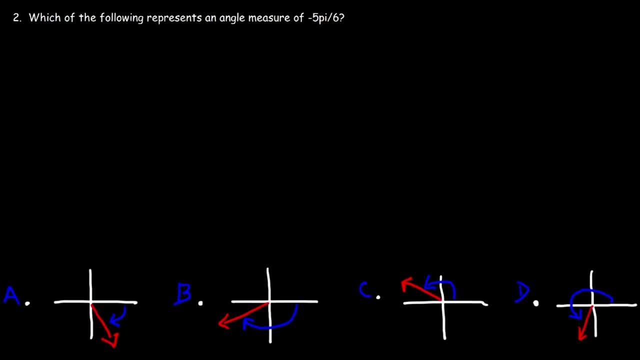 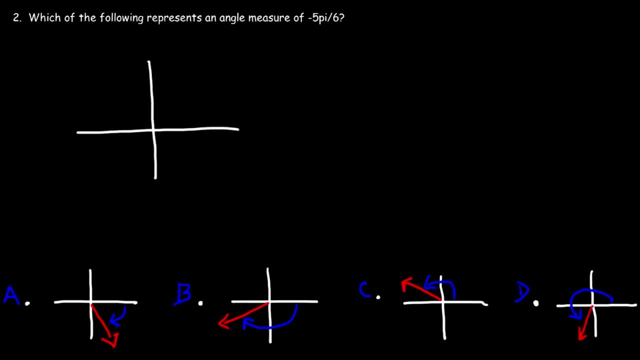 Well, first let's go over the angles that you need to know. This is 0 degrees, 90,, 180,, 270.. Now you can deal with negative angles. So if you're going in, let's say, the counterclockwise direction, the angle measure is positive. Now, if you travel in, 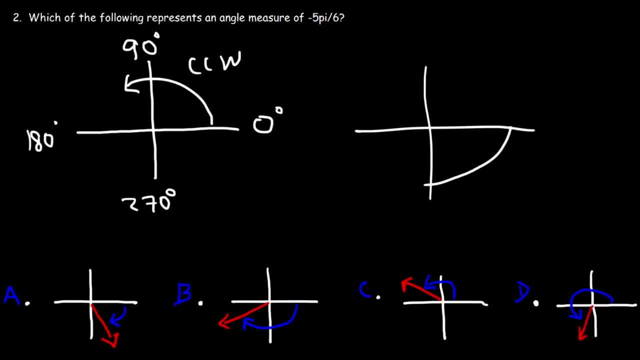 the clockwise direction, the angle measure will be negative. So in this case this is: 0 degrees: 180, 270.. Negative 90, negative 180, negative 270 if you're traveling in that direction. So what we need to do is convert radians to degrees. Let's do that first, So we have negative. 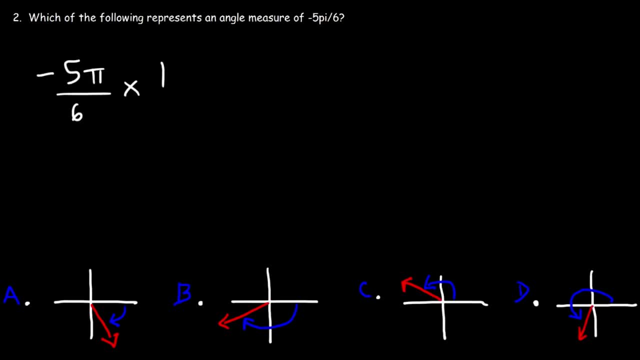 5 pi divided by 6.. So we need to multiply it by 180 divided by pi. So you want to do it in such a way that pi cancels. So we're left with negative 5 times 180 divided by 6.. Now we know that 18 is three times 6.. So we could say that 180 is 6 times 30.. 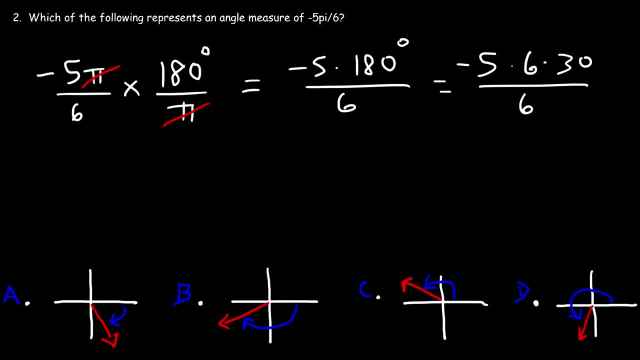 And so we can cancel a 6.. Negative 5 times 30 is negative 150.. So that's the angle. So this is 0, negative 90, negative 180.. So, traveling in the clockwise direction, Negative 150 should be somewhere in this region. 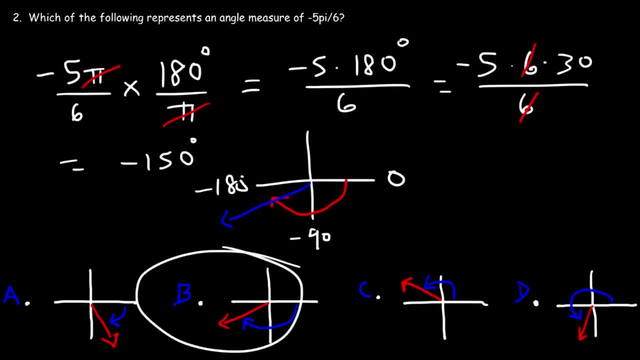 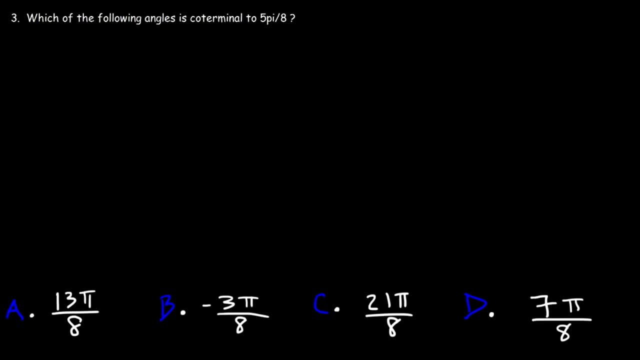 Therefore, we can see that B is the right answer for this problem. Number three: which of the following angles is coterminal to 5 pi over 8?? Now, before we can find the answer, we need to know what a coterminal angle is. 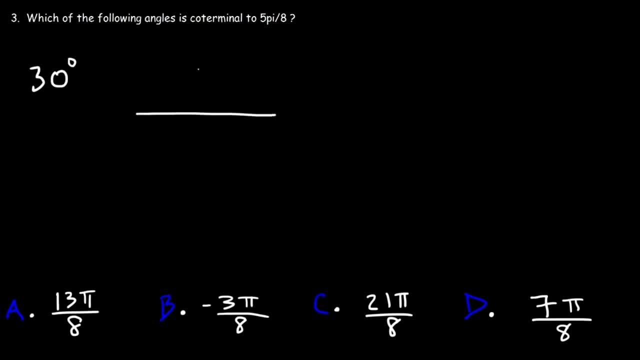 So let's take 30 degrees, for example. So 30 degrees is located in quadrant 1.. So this is quadrant 1, quadrant 2, quadrant 3,, quadrant 4.. A coterminal angle is one in which it's going to land in the same position as the 30 degree angle. 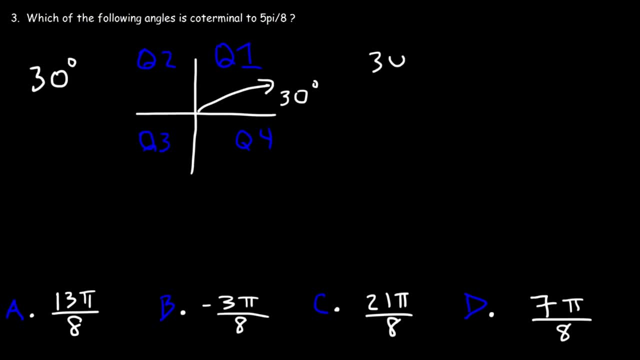 That is in quadrant 1.. And to find a coterminal angle you can either add or subtract 360 to it. If you add 360, you're going to get 390.. So 390 is coterminal to 30.. 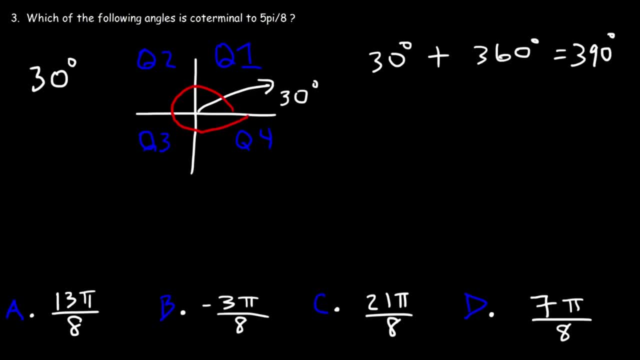 So this is 90, 180, 270, 360, 390.. So you land in the same position. Now, if we did 30 minus 360, this will give us negative 330, which is also coterminal to 30.. 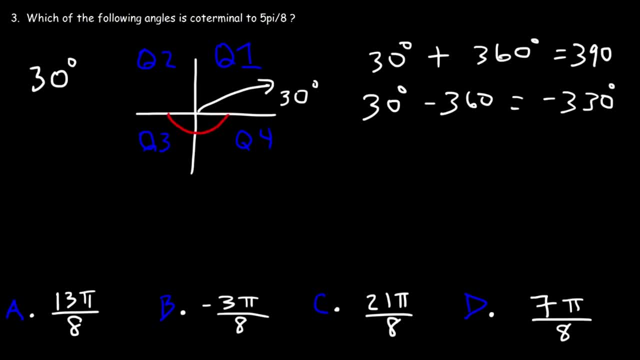 So, starting from here, this is going to be negative 90, negative 180, negative 270, negative 330.. So these angles are coterminal because they have the same position in this graph. So now let's focus on the problem. 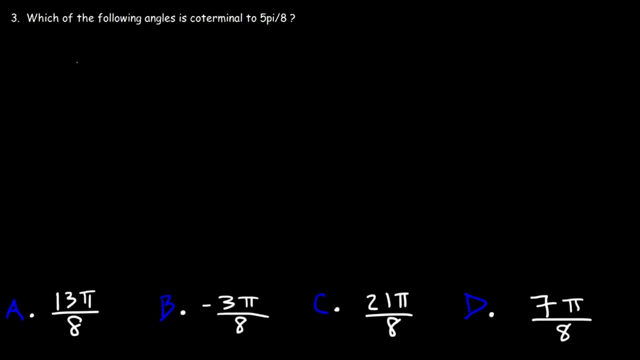 Which of the following angles is coterminal to 5 pi over 8?? So there's two ways in which we can get the answer. We can add 2 pi or we can subtract by 2 pi. So let's start by adding 2 pi. 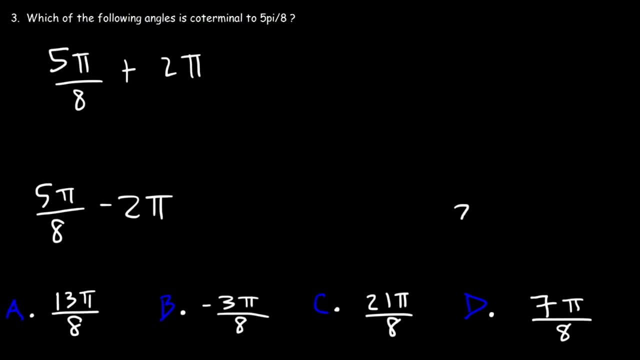 Now keep in mind the reason why we're using 2 pi is because we have the angle and radians, And it's important to understand that 2 pi is equal to 360 degrees. Pi is equal to 180 degrees, So let's turn this into a fraction. 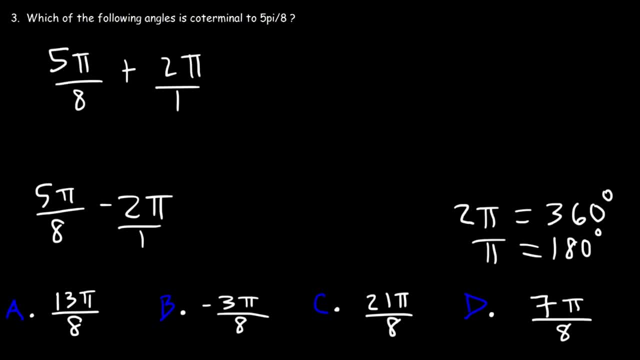 And we need to get common denominators. So we have an 8 on the left side. So we need to multiply the top and the bottom by 8.. So this is going to be 5 pi over 8.. And then 2 pi times 8, that's 16 pi. 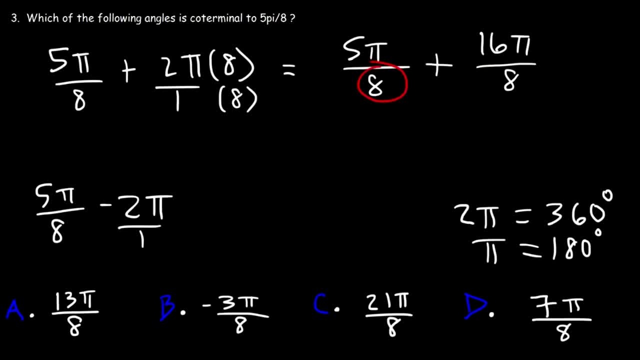 So now that we have the same denominator, we can add the numerators. So 5 pi plus 16 pi is 21 pi. So this is one answer which we do have. So c is the correct answer. 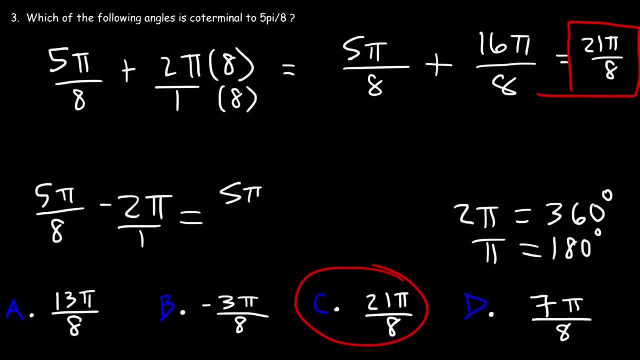 Now, if we subtract it by 2 pi, this is going to be 5 pi over 8.. Well, first we need to multiply this value by 8 over 8.. I'm getting ahead of myself. So this is going to be 5 pi divided by 8, minus 16 pi over 8.. 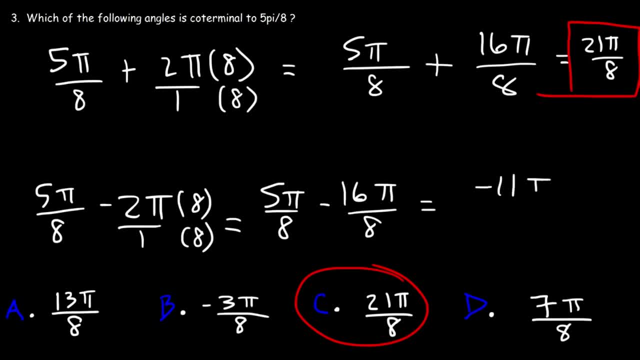 And 5 minus 16 is negative 11. So negative 11 pi over 8 is also coterminal to 5 pi over 8.. So the other answers, a, b and d: they're not coterminal to 5 pi over 8.. 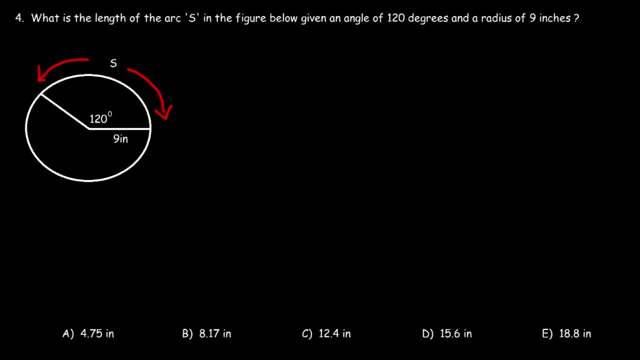 Number 4.. What is the length of the arc s in the figure below, given in a Angle of 120 degrees and a radius of 9 inches? So the formula that we need to get this answer is this: The arc length is equal to the angle in radians. 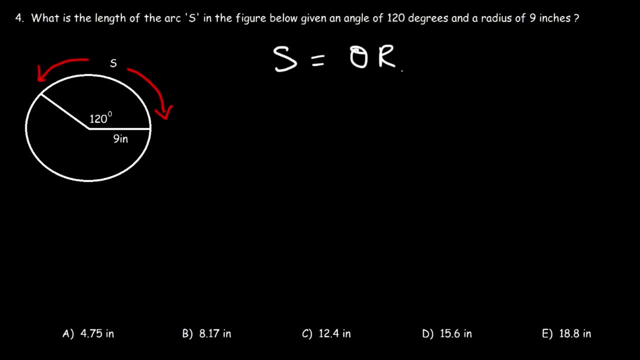 multiplied by the radius of the circle. Now we have the angle in degrees, So we need to convert it to radians. So we have 120 degrees and we need to multiply by pi divided by 180.. So we can cancel the degree symbol. 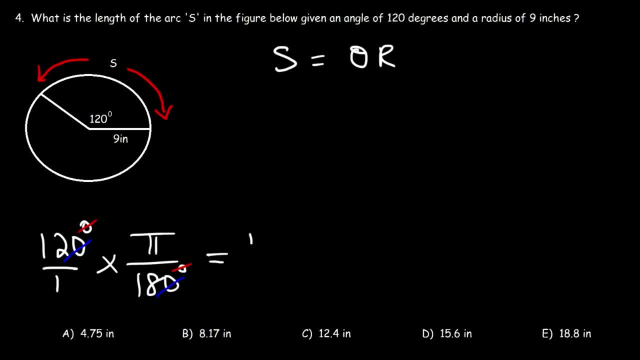 and we can get the radius of the circle. So we have 120 degrees and we need to multiply by pi divided by 180.. We can cancel a 0. So this is equal to 12 pi divided by 18.. 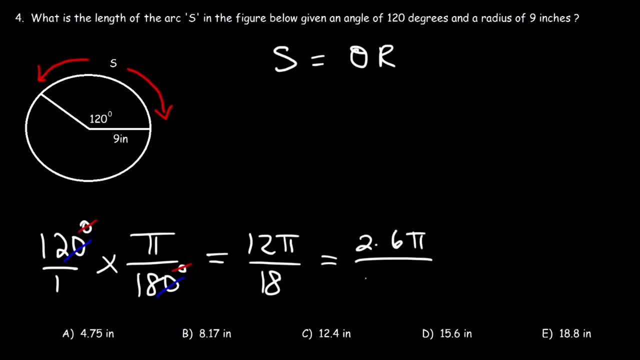 And 12 is 2 times 6. I mean 18 is 3 times 6.. And so we can cancel a 6.. And so the angle in radians is 2 pi divided by 3.. So the arc length is going to be 2 pi over 3. 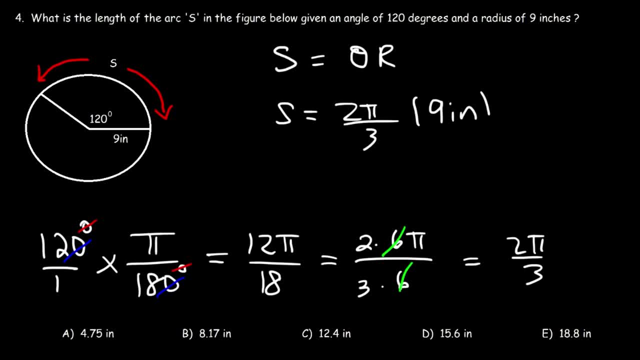 multiplied by a radius of 9 inches- Now 2 times 9- is 18.. and 18 divided by 3 is 6.. So the arc length is 6 pi. Now pi is 3.14159.. So if you multiply 6 by, 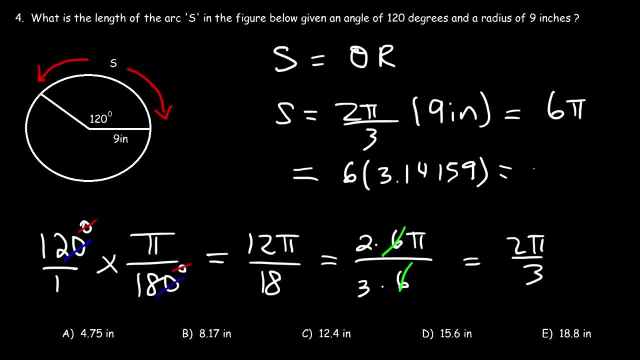 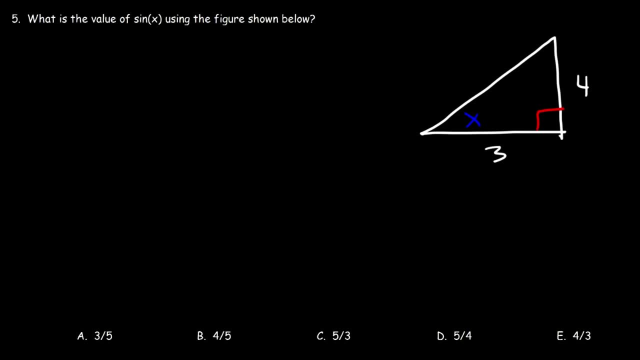 that number. this will give you 18.84954.. So we can round that and say it's 18.8 inches. So e is the answer Number five. what is the value of sine x using the figure shown below? So go ahead and try this problem. Now. the first thing we need to do is we need to find the missing. 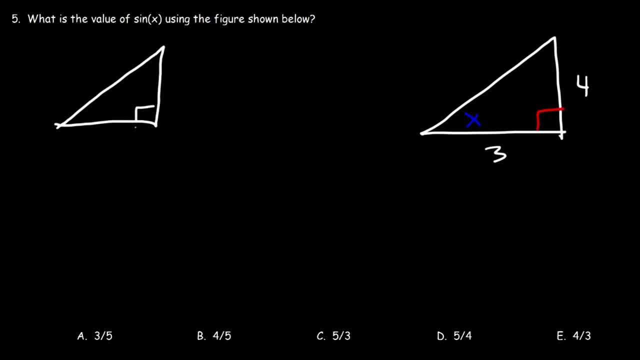 side, And so we have a right triangle. Let's call this a, b and c. So we got to find c, the side length of the hypotenuse, And so we could use the Pythagorean theorem: c squared is equal to a squared plus b squared, So a is 3, b is 4,. 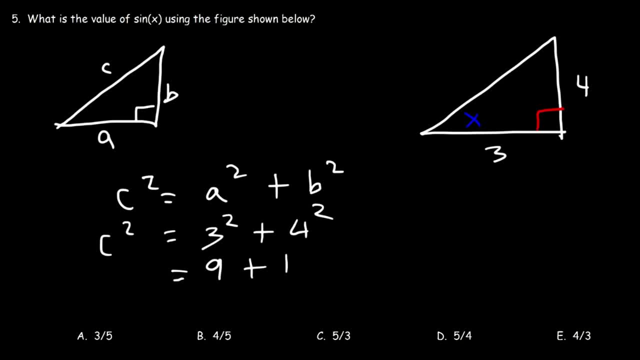 and we need to calculate c: 3 squared is 9,, 4 squared is 16.. And 9 plus 16 is 25.. So now we need to take the square root of 25, which is 5.. So what we have is the 3,, 4, 5 right triangle. 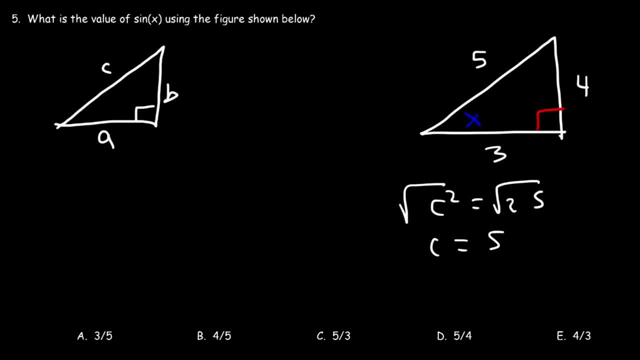 Now there are some special triangles that you want to keep in mind. The 3,, 4, 5 triangle is simply one of them. Here are the other ones. So, in addition to this, there's also the 5,, 12,, 13. 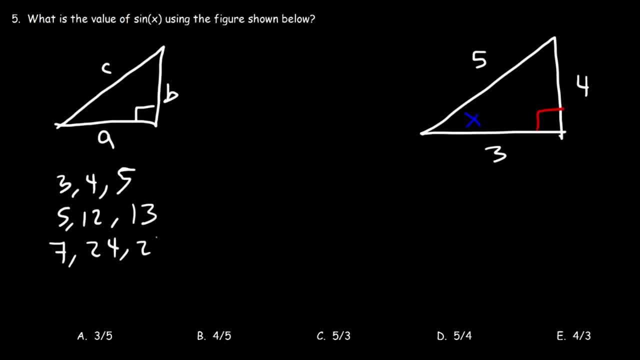 triangle, There's the 7,, 24,, 25 triangle And there's the 8,, 15,, 17 triangle. Now, any ratio of these numbers will also work. For example, if I multiply the 3,, 4, 5 triangle by 2,, I get the 6,. 8,, 10, and 11.. So I get the 6,, 8,, 10, and 11.. So I get the 6,, 8,, 10, and 11.. So I get the 6,, 8,, 10,. 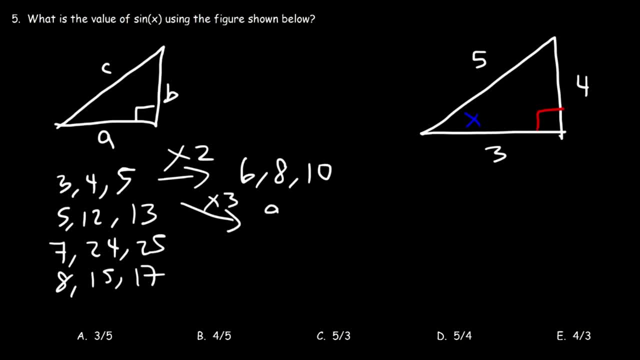 and 11 triangle, Or if I multiply it by 3,, I get the 9,, 12, 15 triangle. So those works as well. Now there are some other triangles that you may see. They're rare, but sometimes you might. 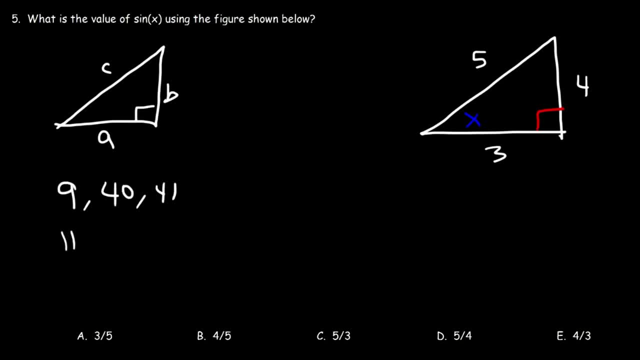 encounter them. There's the 9,, 40, 41 triangle, And I've seen the 11,, 60, 61 triangle. In case you want to write those down Now, you need to be familiar with something called SOHCAHTOA. So what does this expression mean? Well, let's focus on the SOH. 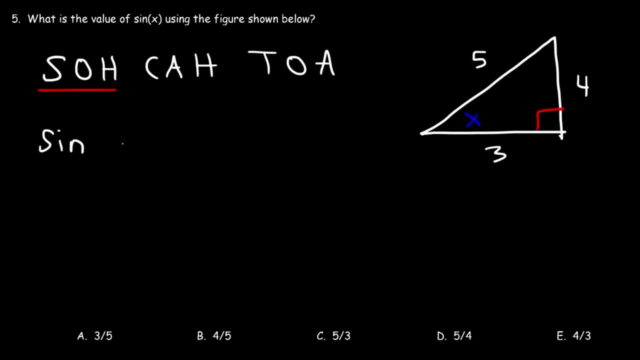 part. S stands for sine, So sine of an angle, it could be theta or it could be. X is equal to opposite divided by the hypotenuse, So that's the sine ratio. O stands for opposite. H is for hypotenuse, So opposite to X is 4.. And adjacent to X is 3.. 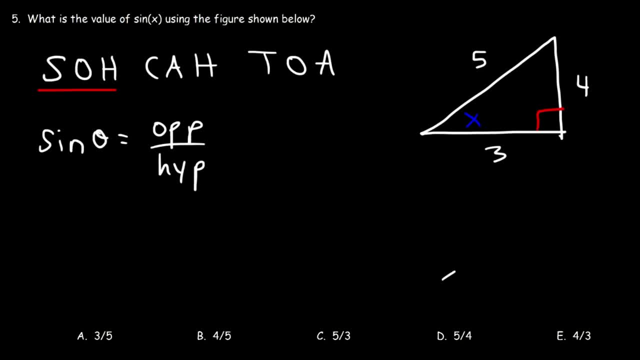 And 5 is the hypotenuse. So let me just show you with a separate triangle. So let's say: this is the angle theta. This is opposite to theta, This is adjacent to it And this is the hypotenuse, which is always across the 90 degree angle. The hypotenuse is the longest side of the triangle. 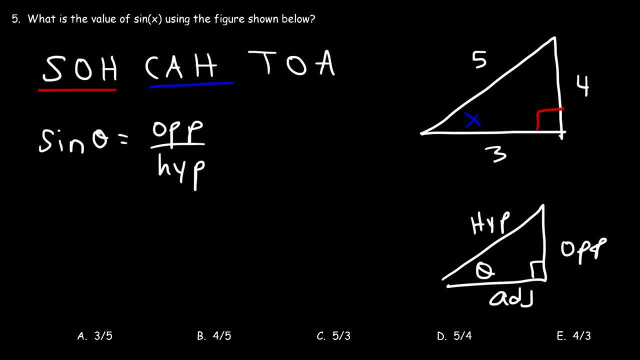 Now the next one: CAH. C stands for cosine. Cosine. theta is the ratio between the adjacent side of the triangle and the hypotenuse. And the last one, tangent, which is associated with TOA. Tangent is the ratio of the opposite. 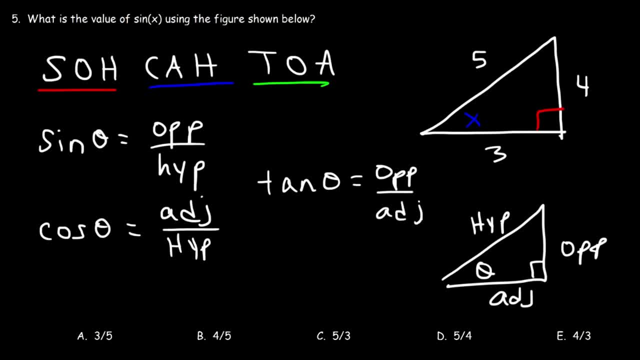 side of the triangle to the adjacent side, And so those are some things that you want to keep in mind, So we're going to use that. So in this example, we want to find the value of sine X. So sine X is going to equal the side opposite to it, divided by the hypotenuse. 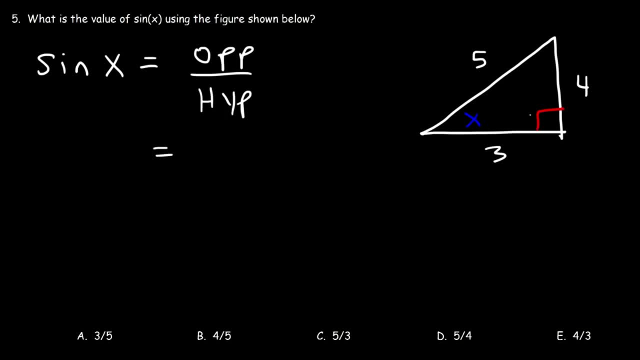 So opposite to X is 4.. And the value of the hypotenuse is 5.. So sine X is equal to 4 over 5.. So therefore B is the right answer in this problem, Number 6.. What is the value of secant X in the? 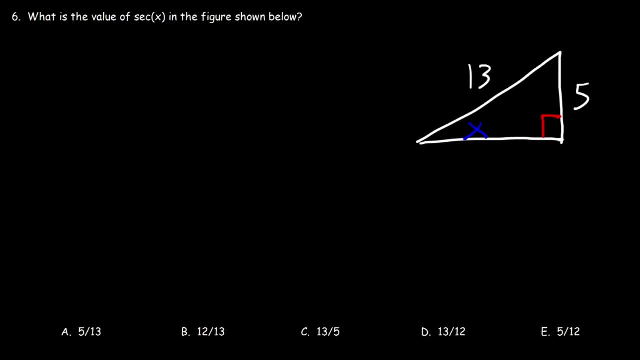 figure shown below. So you need to be familiar with the reciprocal identities. For instance, cosecant is 1 over sine, Secant is 1 divided by cosine And cotangent is 1 over tangent, And it's important to know that tangent is also equal to sine over cosine. So those are some formulas that you may want. 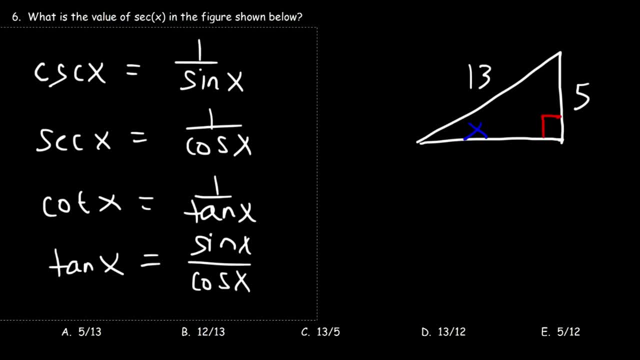 to add to your list. So in this case, to find the value of secant first we need to find the value of cosine. So using SOHCAHTOA, we know that cosine is equal to the adjacent side divided by the hypotenuse. 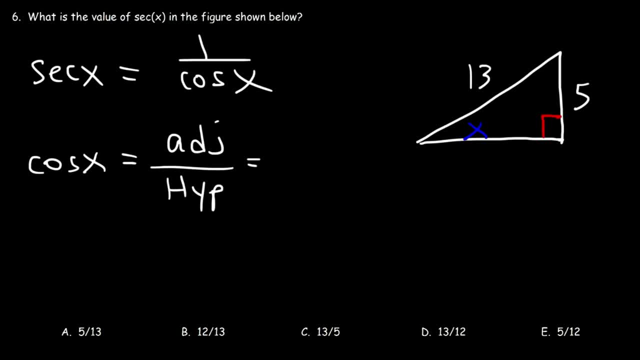 So first we got to find the missing side. Now, what type of triangle do we have? Is it a 3-4-5 triangle, Is it a 7-24-25 right triangle, Or is it a 8-15-17 triangle? 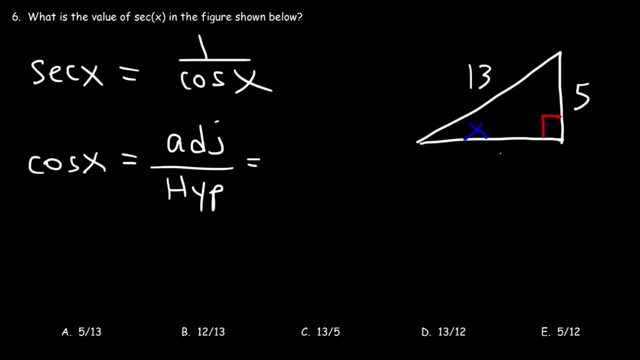 Is it a 9-40-41 triangle Or is it an 11-60-61 triangle? This triangle is the 5-12-13 triangle, And so that's the missing side, And if you ever forget, you can always use this formula. 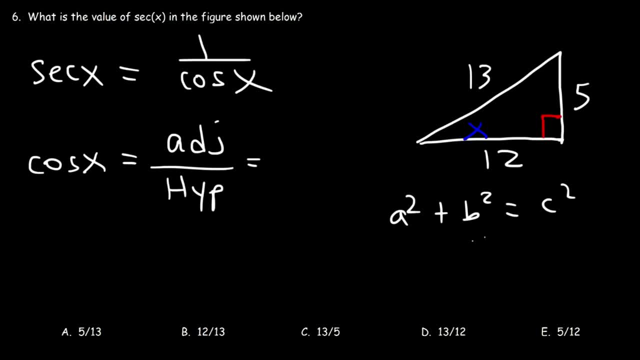 A squared plus B squared is equal to C squared. So A can be any one of these numbers. So let's say A is 5. And we wish to calculate the value of B. Let's say C is 13. So C is 13.. 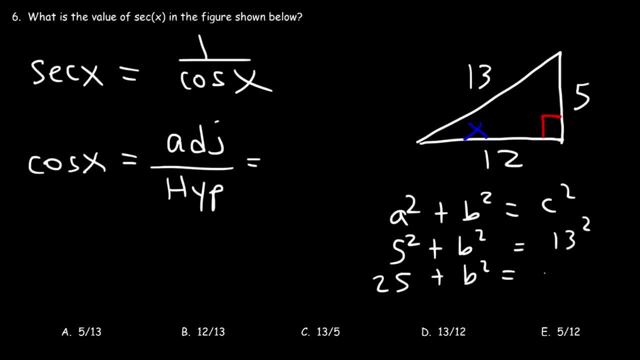 And we wish to calculate the value of B. So let's say C is 13.. So let's say C is 13.. 5 squared is 25.. 13 times 13 is 169.. Now 169 minus 25 is 144.. 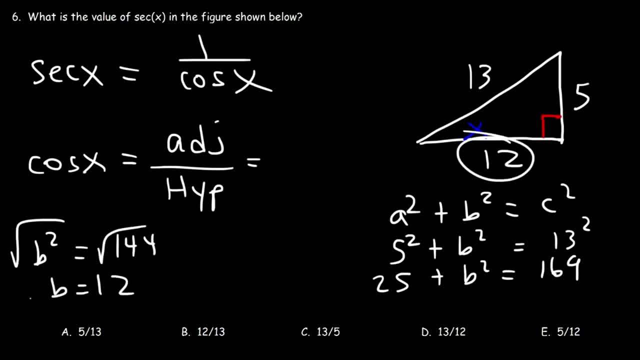 And the square root of 144 is 12.. So you can always find the missing side using this formula if you ever forget the special right triangles. So you can always find the missing side using this formula if you ever forget the special right triangles. 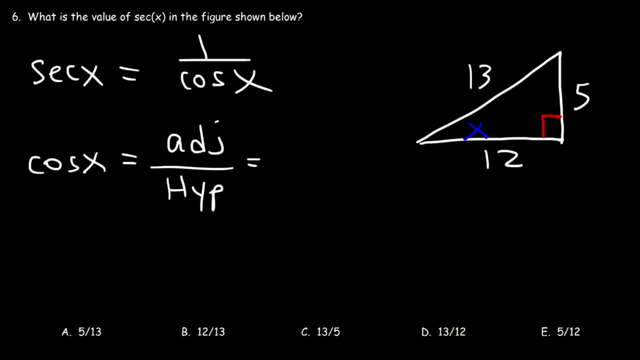 So you can always find the missing side using this formula if you ever forget the special right triangles. Now let's focus on finishing this problem. So adjacent to X is 12 and the hypotenuse is 13.. So it's 12 over 13.. 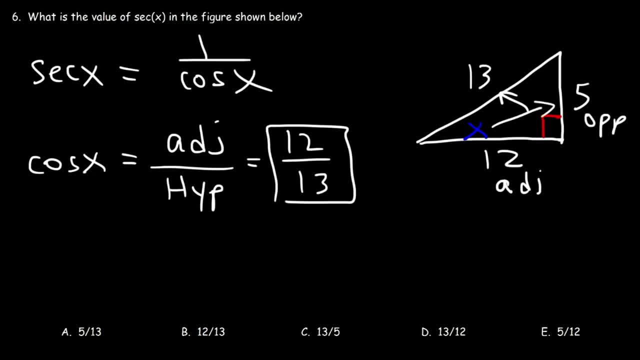 Keep in mind, 5 is opposite to the angle X. So now we have the value of cosine, But our goal is to calculate the value of secant. So secant, which is 1 over cosine, that's 1 over 12 divided by 13.. 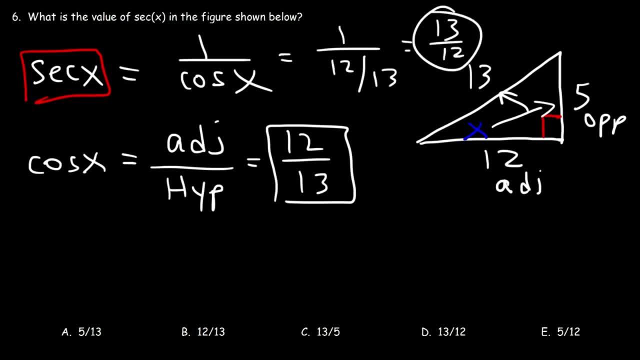 Which is 12 over 13.. 13 over 12.. So the correct answer is answer choice D. Now, if you wish to understand how this works, here's one way in which you can simplify it. So, once you have this, multiply the denominator of. 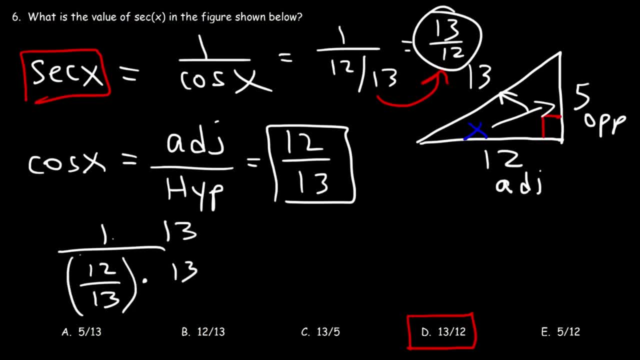 the fraction by 13 and multiply the numerator by 13.. So on the bottom these will cancel, and so on the top of the fraction you're going to have 1 times 13, which is 13, and on the bottom you have 12 left over. So you get 13 over 12, which means that answer choice D is the correct answer to this. 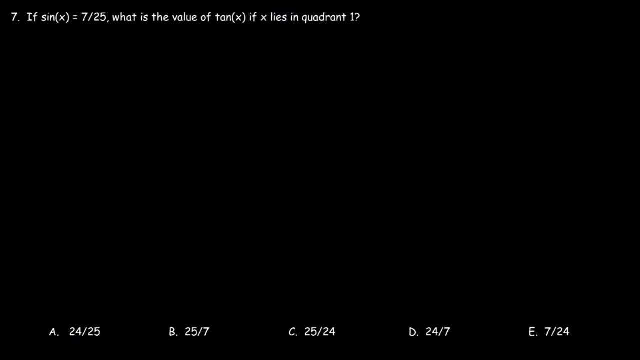 problem Number 7.. If sine x is equal to 7 over 25, what is the value of tangent x if x lies in quadrant 1?? So first let's draw a graph. Now keep in mind: this is quadrant 1,, quadrant 2,, quadrant 3,. 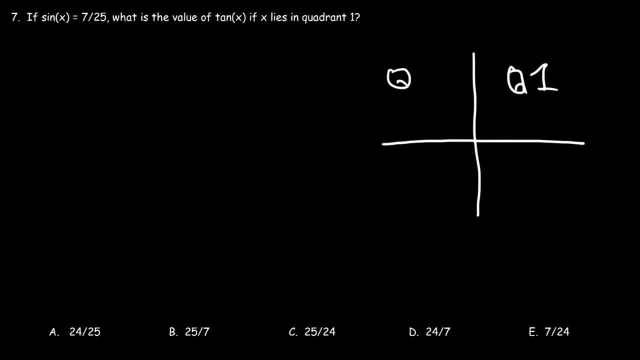 quadrant 4.. So what we need to do is draw a right triangle in quadrant 1, since that's where the angle is located in. So this is going to be x. Now, sine x is 7 over 25 and we know that sine is equal to the opposite side divided by the hypotenuse. So opposite to x is: 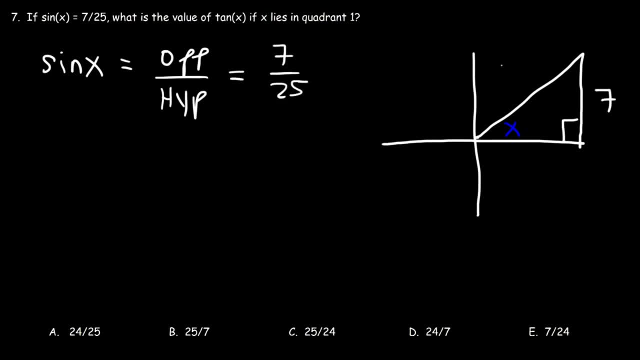 7, because sine is equal to 7 over 25 and the hypotenuse is 25.. Now what type of right triangle do we have? It's not a 5-12-13 or 3-4-5 triangle, It's the 7-24-25 triangle, So the missing side is 24.. So now we can. 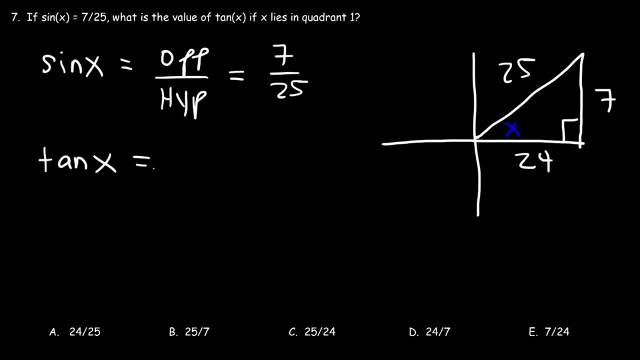 calculate the value of tangent x. So, based on SOHCAHTOA, tangent is equal to the opposite side divided by the adjacent side. So opposite to x is 7 and adjacent to it is 24.. So tangent is 7 over 24. 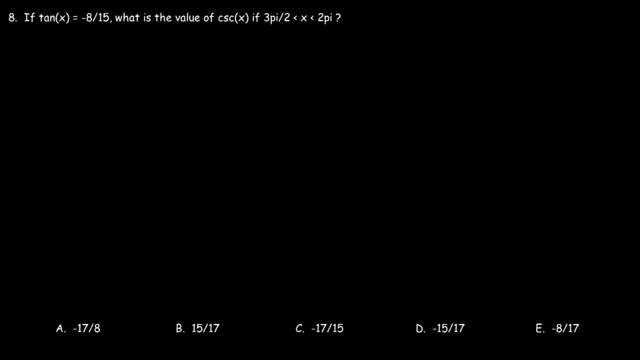 which means that E is the right answer, Number 8.. If tangent x is negative, 8 over 15, what is the value of cosecant x? if x is between 3 pi over 2 and 2 pi, So this is 0. This is 90 degrees, which is pi over 2.. 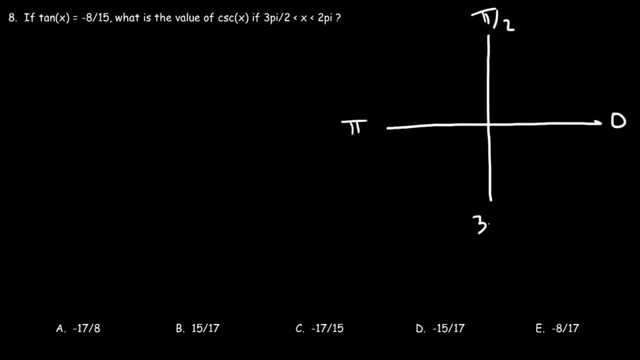 This is pi, that's 180 degrees, and 3 pi over 2 is 270.. 2 pi is coterminal to 0 degrees, which is the same as 360 degrees. So x lies somewhere in quadrant 4 between 3 pi over 2 and 2 pi. So therefore we need to draw a. 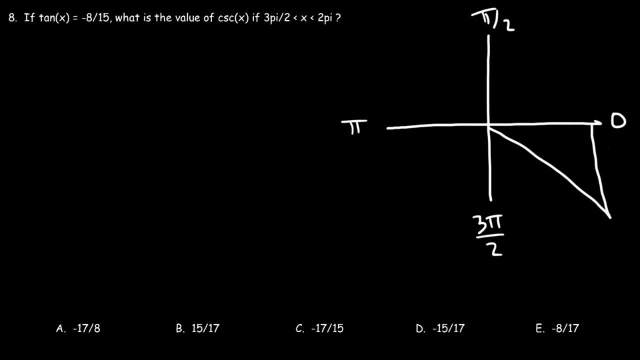 triangle in quadrant 4.. Now x is a large angle and so x is measured from the positive x-axis. Now it's going to create a reference angle which we'll call theta. Now we can use the reference angle to calculate the value of tangent x. So we're going to use the reference angle to calculate the value of tangent x. 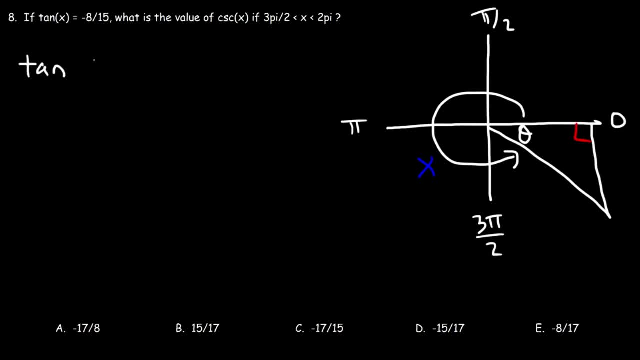 Now tangent is associated with the opposite side divided by the adjacent side, And so tangent in this example is negative 8 over 15.. So opposite to theta, that's going to be negative 8 and the adjacent side is 15.. Now this makes sense. 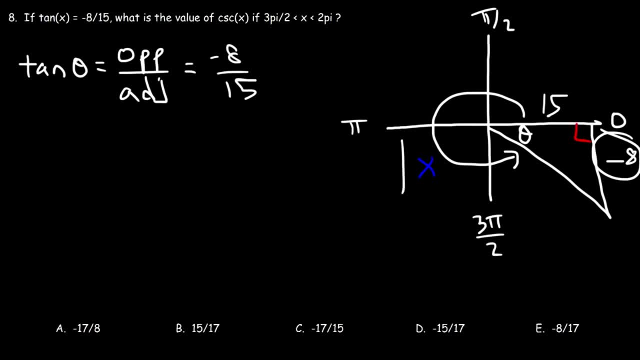 why this is negative? because it's going in the negative y-direction. The 15 is along the positive x-axis, so that's going to be positive 15.. So here we're dealing with the 8,, 15, 17 triangle. So now we can calculate the. 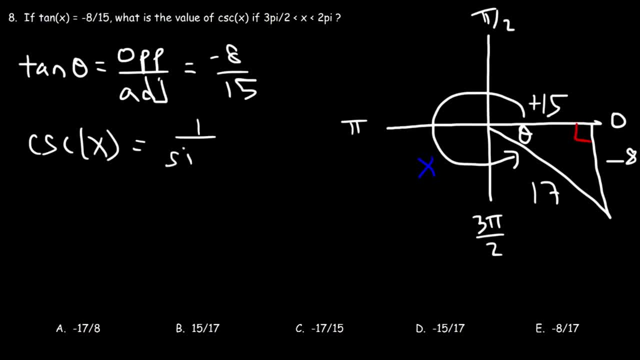 value of cosecant x. Cosecant is 1 over sine and sine x is going to be the opposite side divided by the hypotenuse. So sine theta, which is going to be the same as sine x in this problem, is equal to the opposite side, which is negative. 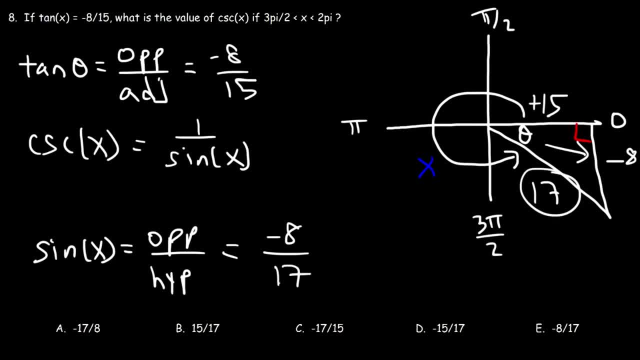 8 and the hypotenuse is negative 8. Cosecant x is 17.. So if sine is negative 8 over 17, cosecant is the reciprocal of that. So it's going to be negative 17 over 8. You just need to flip the fraction. 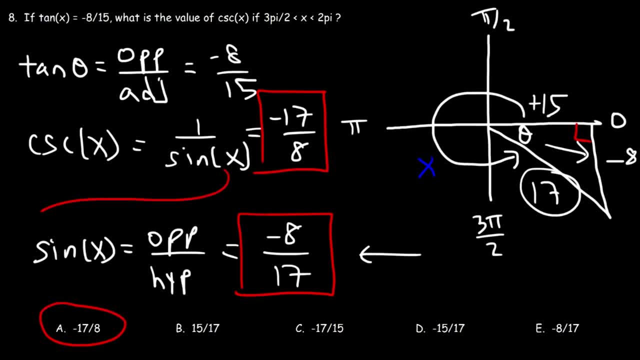 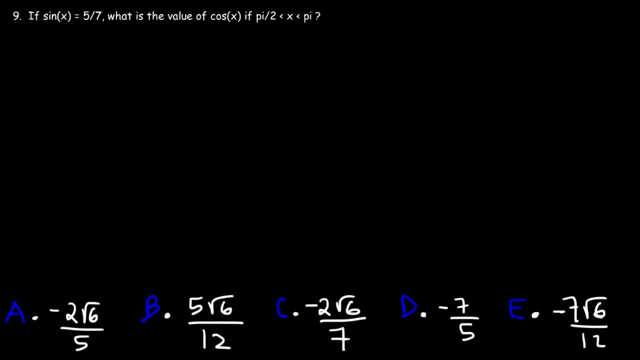 So the answer is this, which correlates to answer choice A, Number 9.. If sine x is equal to 5 over 7, what is the value of cosine x if x is between pi over 2 and pi? So I'm going to use the Pythagorean identities to get the answer for this problem. 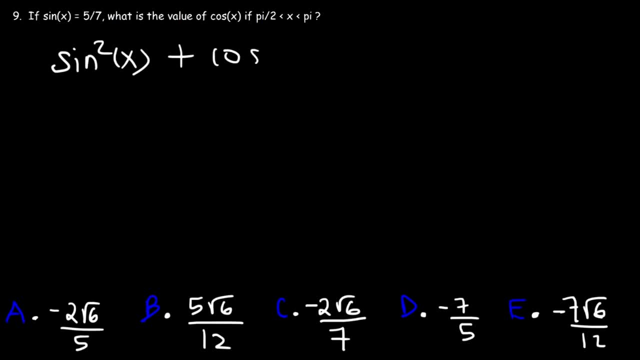 You need to know that sine squared plus cosine squared is equal to 1.. Now there are some other identities that you need to be familiar with. Another Pythagorean identity is this one: 1 plus cotangent squared is equal to cosecant squared, and also 1 plus tangent squared is equal to secant squared. So make sure you 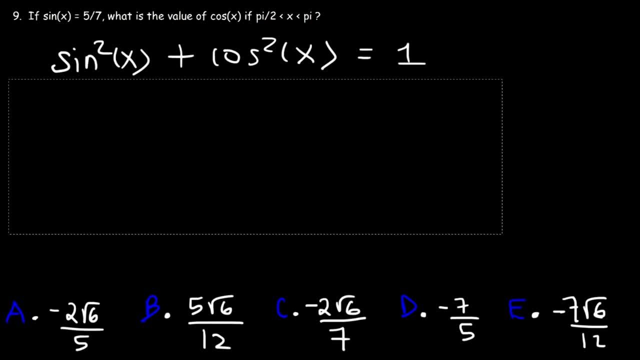 know these three Pythagorean identities. Now let's replace sine with 5 over 7 and let's calculate the value of cosine: 5 squared is 25.. 7 times 7 is 49. And I'm going to replace 1 with 49 over 49, because 49 divided by 49 is 1 and I need to. 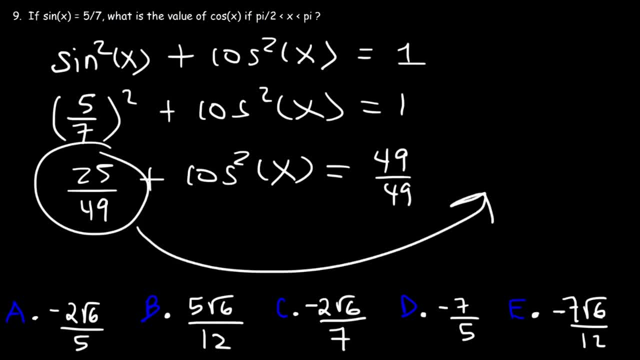 get common denominators. So I'm going to move this. I'm going to move it to the other side. So 25 over 49 is positive on the left, but it's going to be negative on the right side. So cosine squared is 49 over 49 minus 25 over 49.. 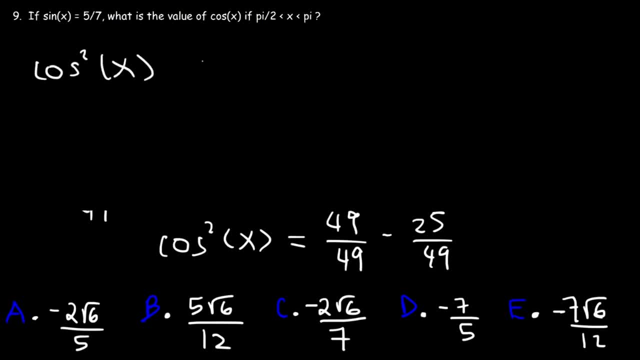 49 minus 25 is 24.. And so cosine squared is 24 over 49.. Okay, Now let's take the square root of both sides. The square root of cosine squared is cosine. The square root of 49 is 7.. 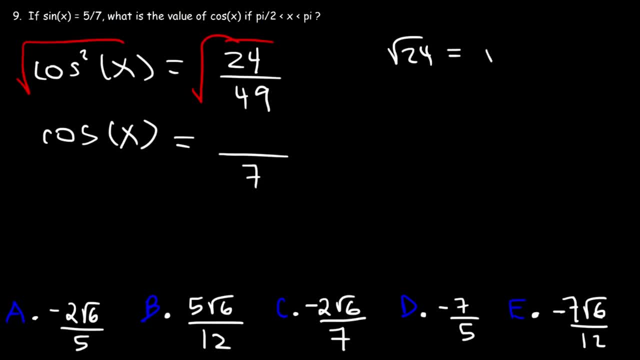 Now we need to simplify the square root of 24.. 24 is 4 times 6. And the square root of 4 is 2.. So the square root of 24 is 2 square root 6., And the answer can be plus or minus. 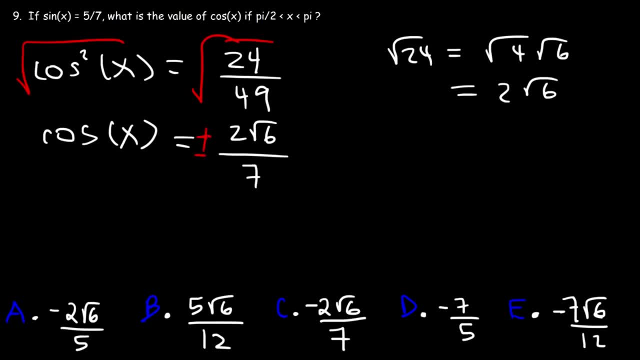 Now, looking at our answer choices, the only one that has 2 square root 6 over 7 is answer choice C. So that has to be the answer. Now what if both answers were present? So what if we had positive and negative 2 square root, 6 over 7?? 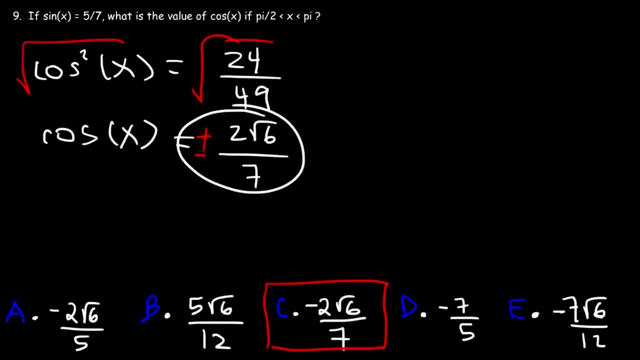 How can we determine which one is the correct answer? Well, for one thing, we have a positive and negative 2 square root- 6 over 7.. So what if we have a positive and negative 2 square root- 6 over 7?? 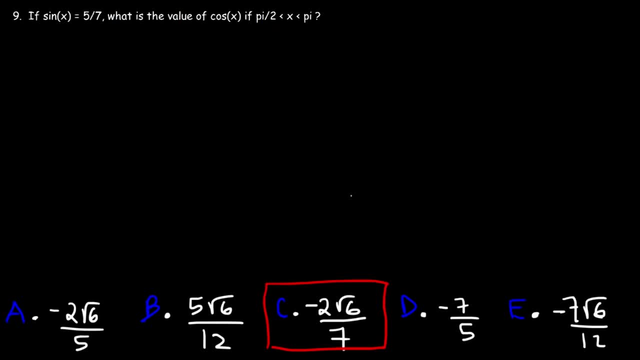 How can we determine which one is the correct answer? Well, for one thing, we have a positive and negative 2 square root, 6 over 7.. 1 will be the answer, And the result is that the sorrow of one of you playing with you atatrains becomes 2.. 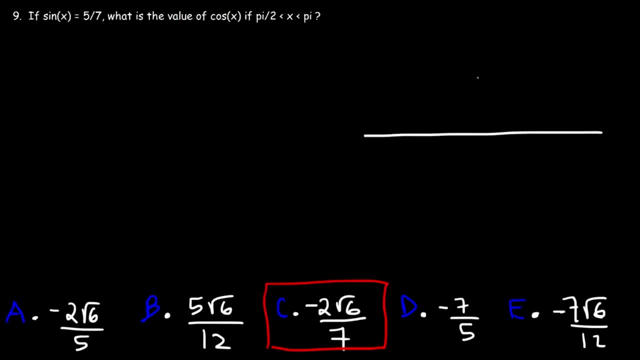 Because the 2 square root 6 over 7.. We will not live to read that letter. The answer is x, The answer is x, The answer is 20.. And we still don't have a positive or negative 2 square root. 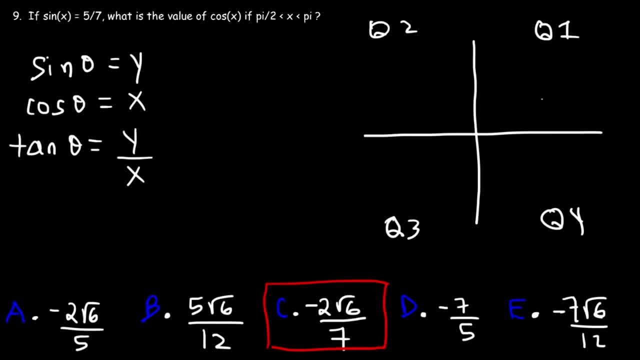 And we still have a negative 2 square root, 6 over 7.. 5 square root: 6 over 7.. that's y divided by x. Now, y is positive above the x-axis. it's positive in the first two quadrants. y is negative below the x-axis. that's it. it's negative in quadrant 3 and 4.. 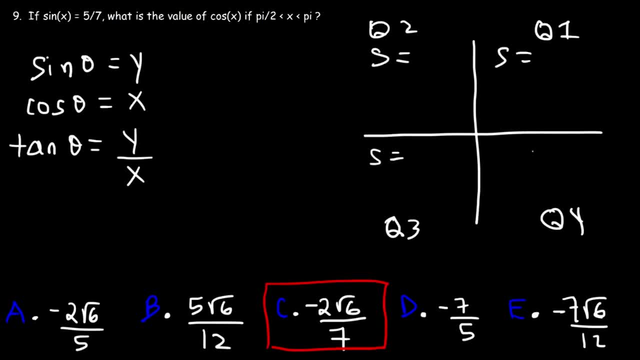 And sine is associated with the y-value. So therefore, sine is positive in quadrants 1 and 2, and it's negative in quadrants 3 and 4.. Now, cosine is associated with the x-value and x is positive on the right side and it's negative on the left side, So cosine is positive. 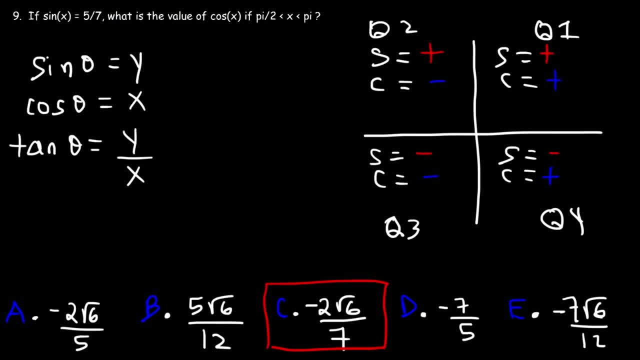 in quadrants 1 and 4, and it's negative in 2 and 3.. Now the last one, tangent is y over x. So therefore tangent is going to be positive whenever sine and cosine have the same sine, That is, they're both positive or both negative. 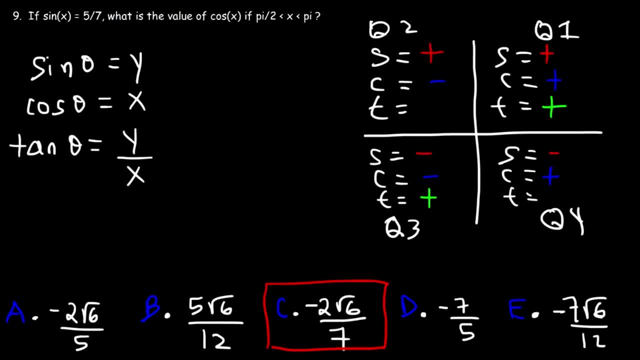 Because a positive divided by a positive is a positive number. A negative number divided by a negative number is a positive number. Now, tangent is negative whenever sine and cosine have opposite signs. If you divide a positive number by a negative number, you're going to get a negative. 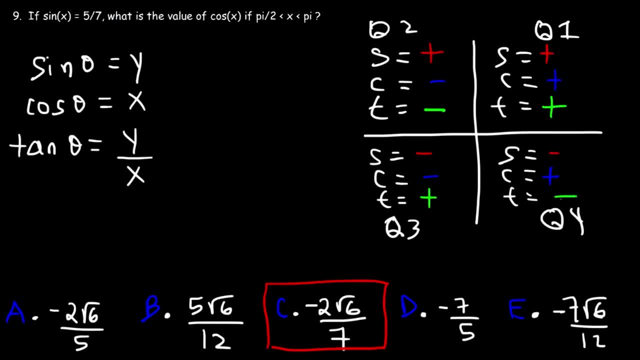 result. Or if you divide a negative number by a positive number, it's still a negative result. So tangent is negative in quadrants 2 and 4, and it's positive in 1 and 3.. So now x is between pi over 2 and pi, So we're dealing with quadrant 2.. And cosine is negative. 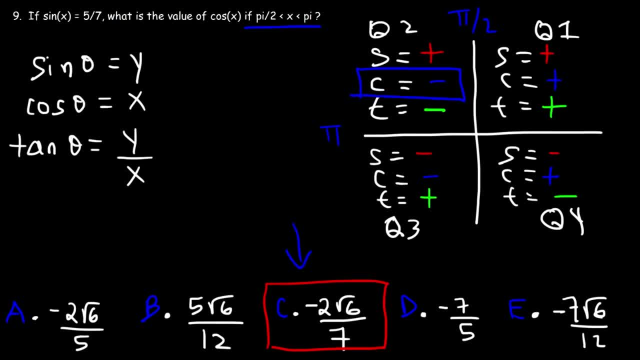 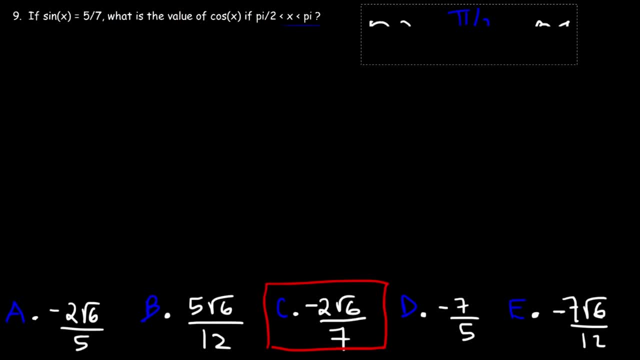 in quadrant 2.. So, therefore, we know that the answer has to be C. Now, for those of you who want to use right triangle trigonometry, as opposed to Pythagorean identities, to solve this problem, here's what you can do. So we realize that x is in quadrant 2.. It's between 90. 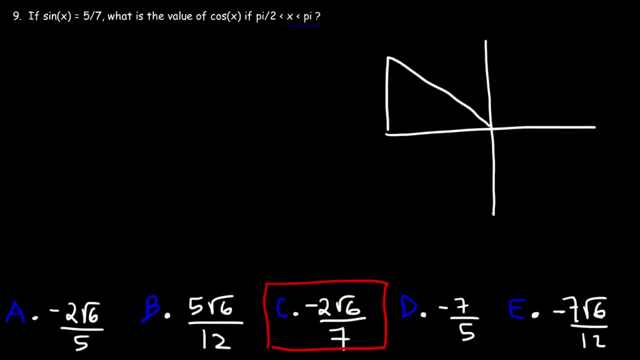 and 180.. So we need to draw the right triangle in quadrant 2.. So that's the value of x. So it's going to form a reference angle. theta: Now we know that sine is equal to opposite sine divided by the hypotenuse, And so sine is 5 over 7.. Opposite to theta is 5, and hypotenuse. 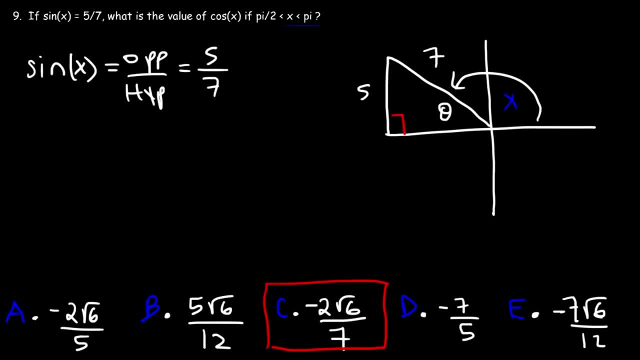 is 7.. So let me draw the right angle. Now we need to find the value of the missing side, So we have to use the Pythagorean theorem to do so. So a squared plus b squared is equal to c squared. We're going to say a is 5, and we're looking for the missing side, b, c is. 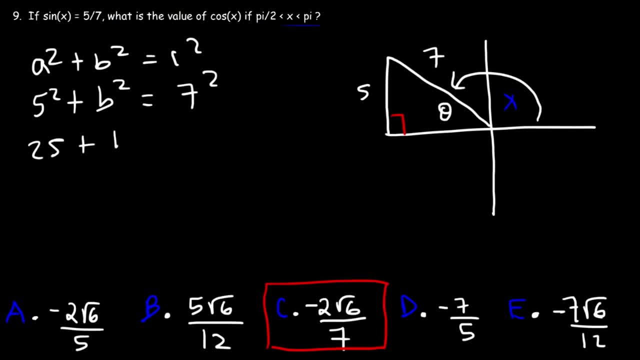 7.. 5 squared is 25, and 7 squared is 49.. 49 minus 25 is 24.. So now we need to take the square root of both sides: 24 is 4 times 6, and the square root of 4 is 2.. So this: 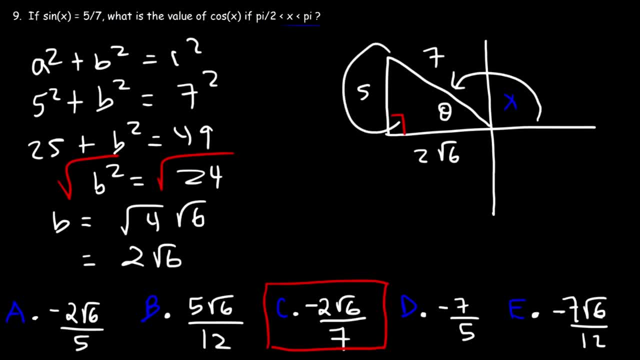 is going to be 2 square root 6.. Now y is positive above the x-axis and x is negative on the left side. So this is going to be negative 2 square root 6.. So now we can calculate the value of cosine. Cosine is equal to the adjacent side which. 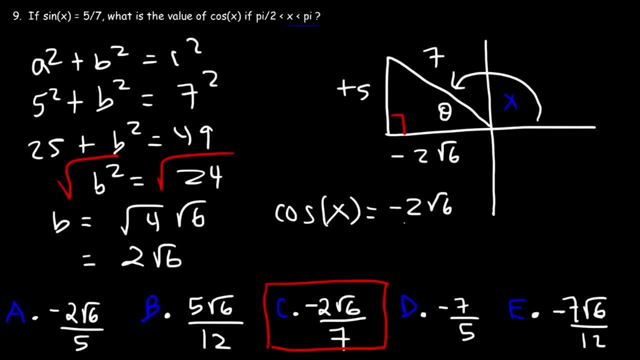 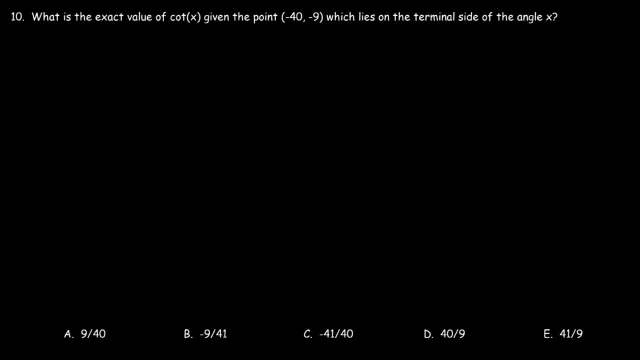 is negative, 2 square root 6 divided by the hypotenuse, which is 7.. So, as you can see, this will give us the same answer, which is answer choice C, Number 10.. What is the exact value of cotangent x, given the point negative? 40 comma negative. 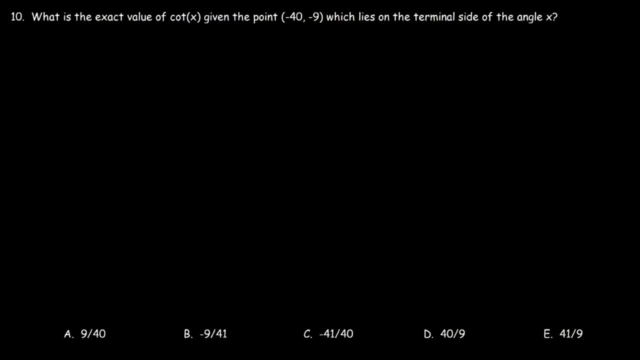 9,, which lies on the terminal side of the angle x. So how can we find the answer And what exactly is meant by the terminal side of an angle? Now, an angle is formed between two rays, So here's the first ray and here's the second. 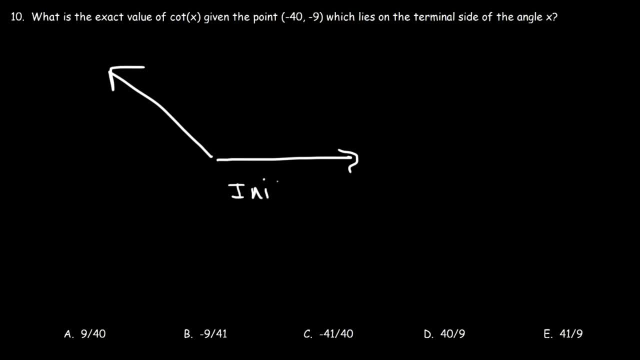 ray. The first ray is known as the initial side. The second ray is called the terminal side And it makes sense why it's called this way, because the angle is measured from the initial side And it ends at the terminal side And it meets at a common endpoint known as the vertex. 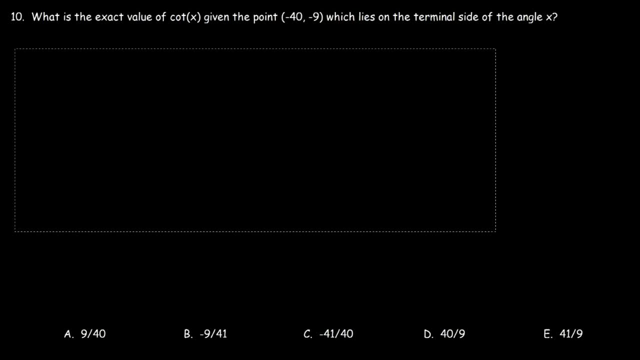 So now you know what the terminal side of an angle is. But how do we use this information to get the exact value of cotangent x? Well, first we need to plot this point. So first we need to travel 40 units to the left, And then we need to go down by 9 units. 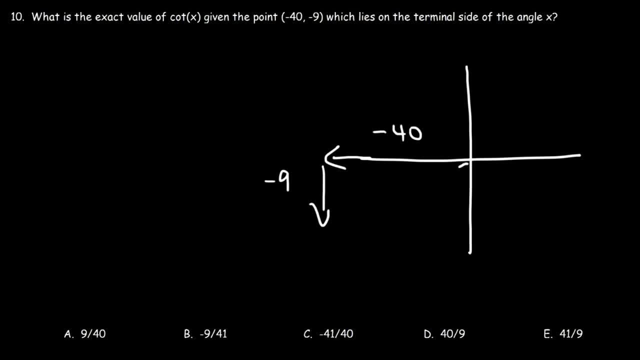 So this is negative 40,, this is negative 9.. And the hypotenuse of this triangle is the terminal side of the angle And along the x-axis we have the initial side. So the angle x is measured from the initial side to the terminal side. So that's x Which I'm going. 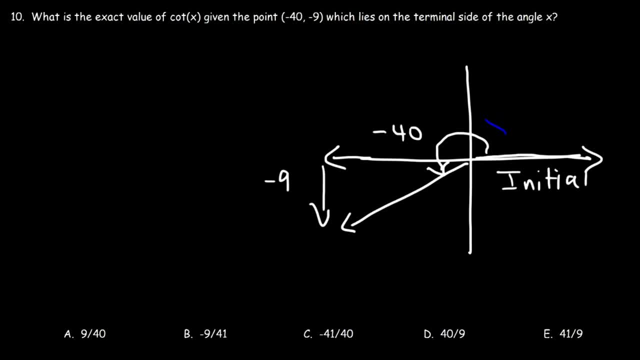 to draw like this. Now this is going to form a reference angle- theta and cotangent x and cotangent theta will give you the same result, so keep that in mind. Now we still have a right triangle, and this is a special right triangle. 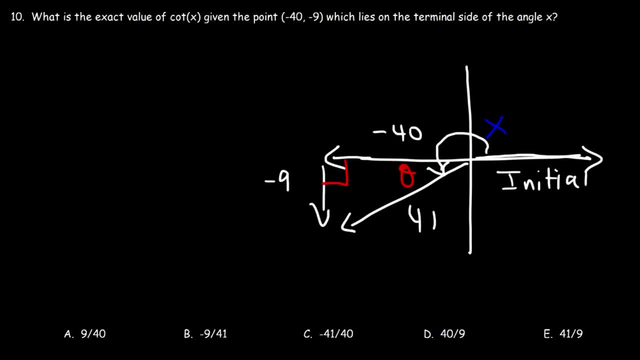 It's the 9,, 40, 41 triangle, so therefore, the hypotenuse is 41.. The hypotenuse is always positive for these types of problems, So now that we've completed the triangle, all we need to do is calculate the value of. 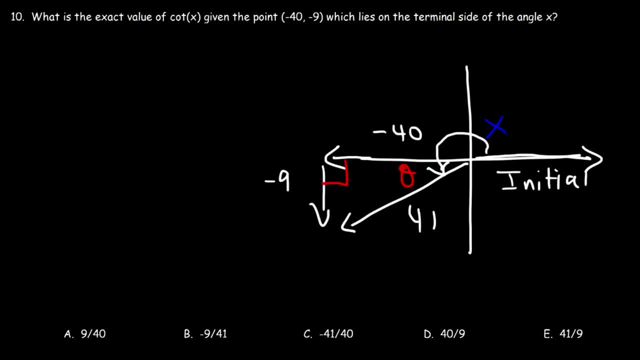 cotangent, But let's find the value of tangent first. Tangent x, which is the same as tangent, theta in this problem is equal to the opposite side divided by the adjacent side. So opposite to theta is negative 9, adjacent to it is negative 40.. 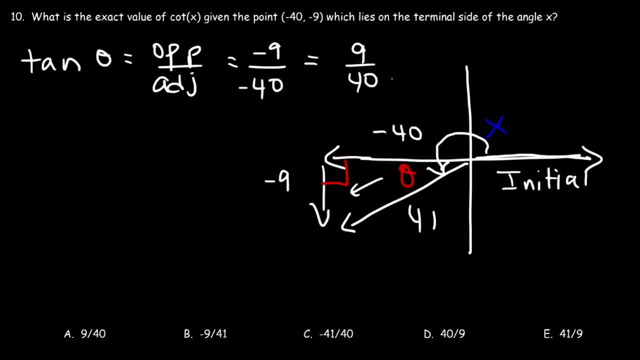 Negative 9 divided by negative 40 is positive 9 over 40. Now cotangent is simply the reciprocal of tangent. So if tangent is 9 over 40. Similarly, cotangent is 40 over 9. So tangent and cotangent are positive in quadrant 3.. 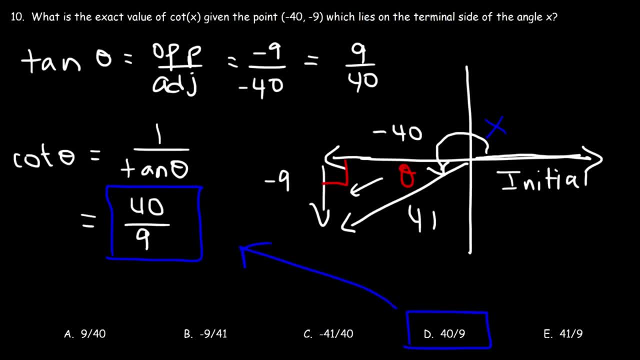 So D is the right answer: 40 divided by 9.. Now, one thing I do want to mention. Now we know that this is the terminal side, so I'm going to write T for terminal side, And when it says that the point lies on the terminal side, the point is actually right. 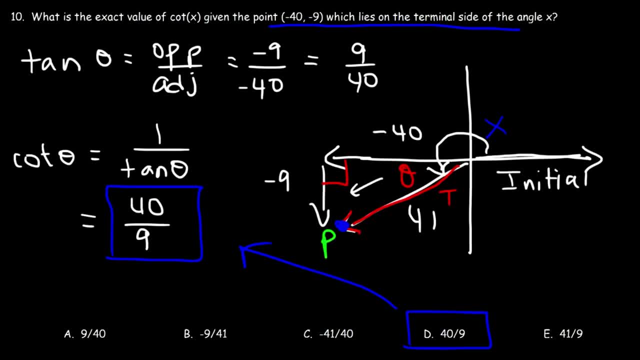 here. This is the terminal side, This is the tangent. This is the point where x is negative 40 and y is negative 9.. So thus you can see why the point lies on the terminal side of angle x. So I just want you to understand the problem visually so you know what to do in order to 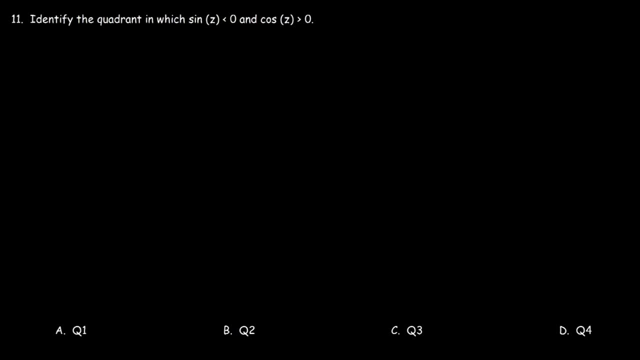 get the answer, Number 11.. Identify the quadrant in which sin z is less than 0 and cos z is greater than 0.. 1.. So the fact that sine z is less than 0 tells us that sine is negative and cosine is positive. 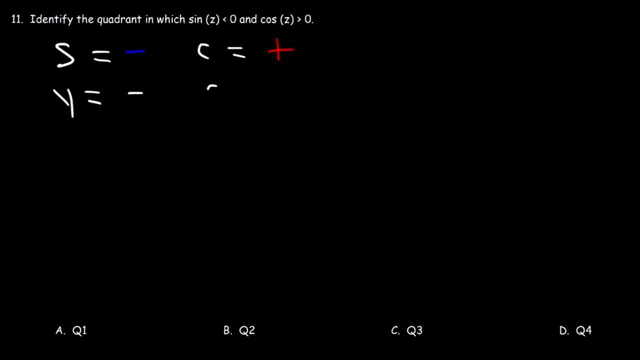 Now, sine is associated with the y value and cosine is associated with the x value, So in which quadrant is x positive and y is negative. So x is positive towards the right, Y is negative as you go down. So therefore we're dealing with quadrant 4.. That's the answer. 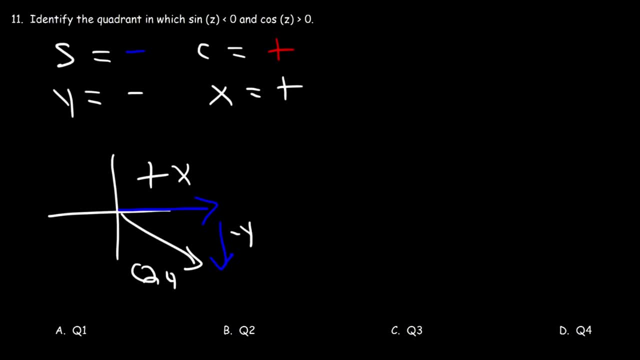 So that's when x is positive and y is negative. Now perhaps you've heard of the expression: all students take calculus. Do you know what that means? What do you think it means? So the first word all tells us that sine is negative. 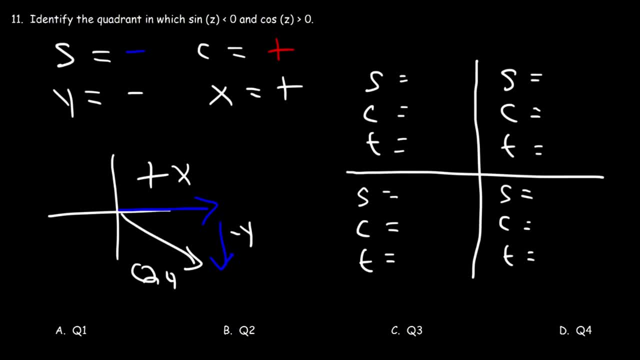 It tells us that everything is positive in quadrant 1. And it goes in order. So all students s for students. so in quadrant 2, sine is positive. Take that means tangent is positive in quadrant 3.. And then calculus, cosine is positive in quadrant 4.. 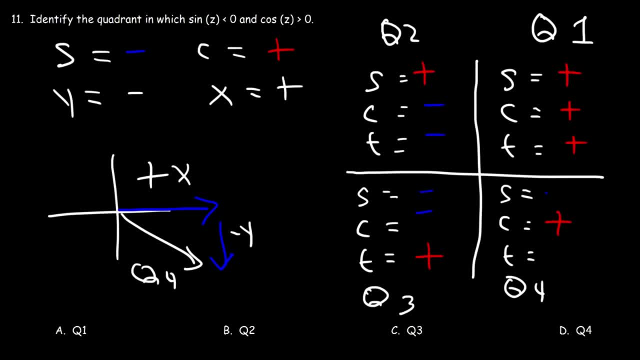 Everything else is negative, And so you can also use that expression to help you remember what's positive and what's negative, if you prefer to do it that way. Sine is negative in quadrants 3 and 4.. Cosine is positive in quadrants 1 and 4.. 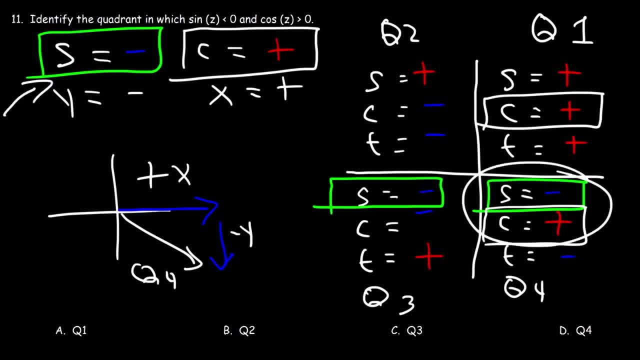 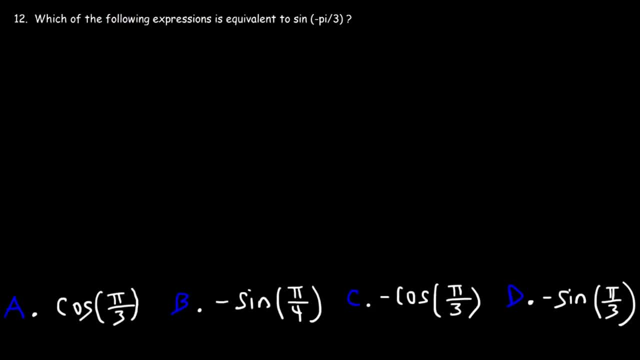 So the answer occurs in quadrant 4.. That's when sine is negative and that's when cosine is positive. So therefore d is the right answer. Number 12, which of the following expressions is equivalent to sine negative pi over 3?? 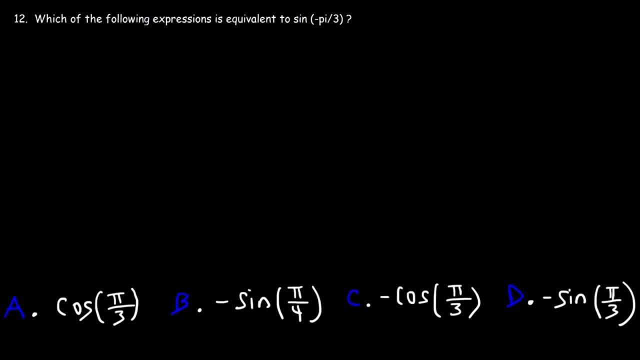 Now, in order to find the answer, you need to be familiar with the even and odd trigonometric functions. By the way, if you need to find more videos on trig, check out my playlist. It's my new trigonometry playlist. 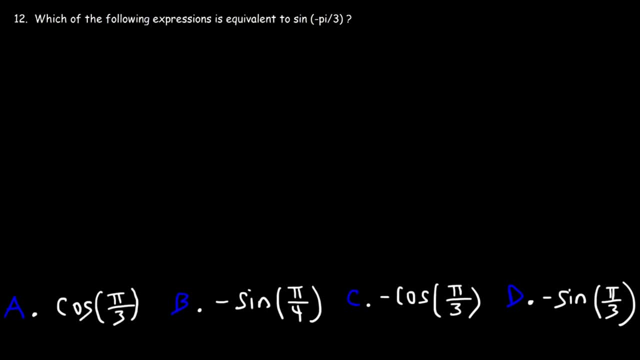 You can search it on YouTube or you can find it in this video. So if you click that button on the right, you should be able to access it. If not, you can check in the description section of this video to find it. 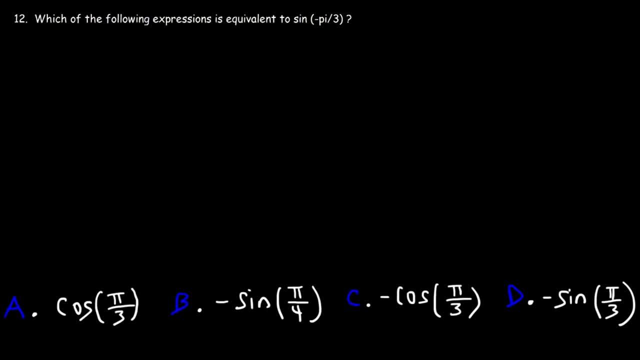 Or at one of the end screens at the end of this video. It should show up at the last 20 seconds of this video, So let's focus on this problem Now. you need to know that sine of negative x is equal to negative sine x. 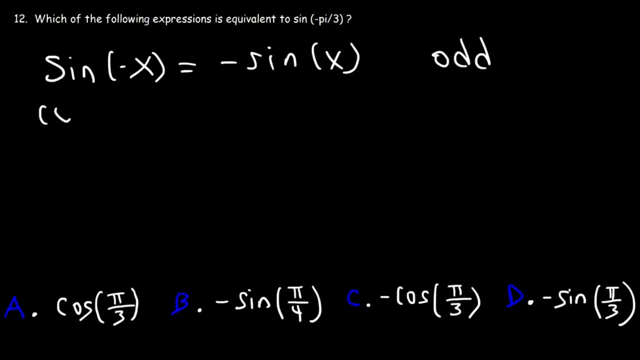 So sine is an odd function. Cosine negative x is equal to positive cosine x, So cosine is an even function Cosecant, which is the reciprocal of sine. that's an odd function, So it's negative cosecant x. 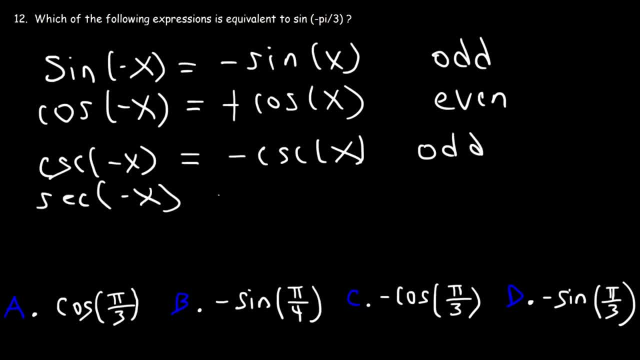 Secant, which is the reciprocal of cosine, is an even function. So secant negative x is the same as secant x. Now the next one is tangent. Tangent is an odd function, like sine, So tan negative x is negative tangent x. 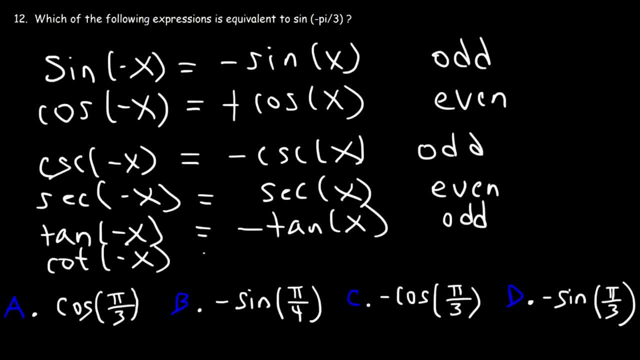 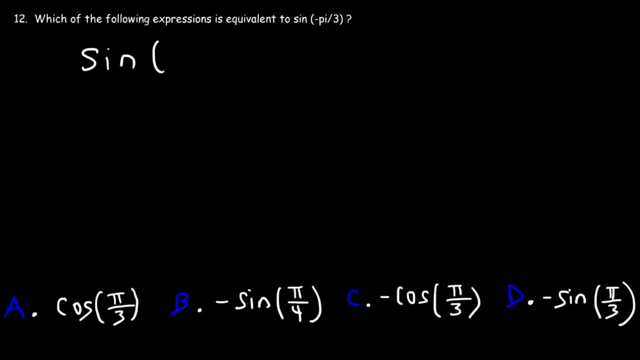 and cotangent is also an odd function. Cotan negative x is negative cotan x. So make sure you know these properties. Now let's go ahead and figure it out ahead and finish this. So we said that sine negative x is equal to negative sine x. So 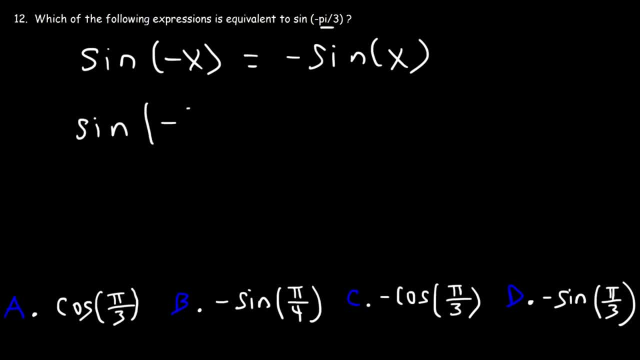 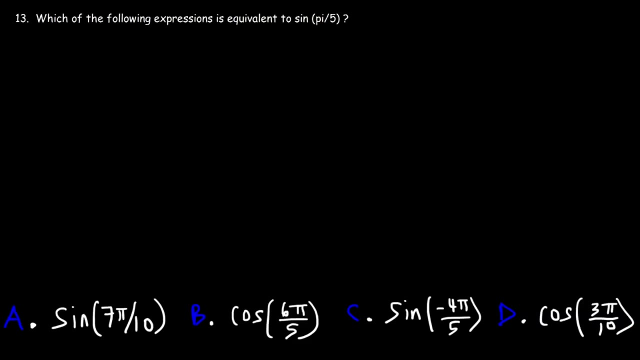 x is going to be pi over 3.. So sine negative pi over 3 has to equal negative sine pi over 3, based on that identity. So therefore, d is the correct answer. Number 13.. Which of the following expressions is equivalent to sine pi over 5?? Now, how can we find the answer? 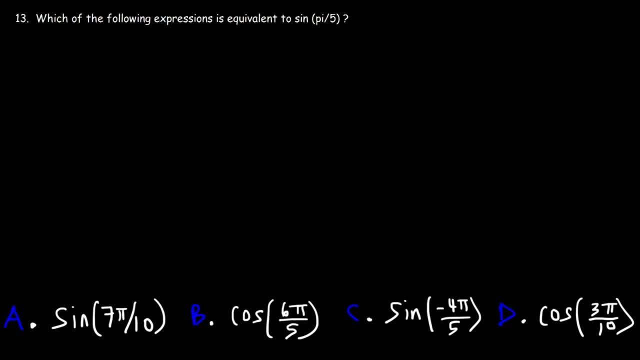 if we don't have access to a calculator. You need to be familiar with the co-function identities. So, for instance, sine theta is equal to the co-function of sine is cosine, So it's cosine 90 minus theta, And cosine theta is sine 90 minus theta. 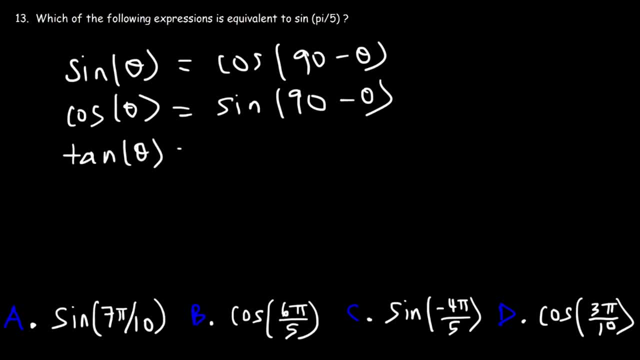 Now tangent theta, the co-function of tangent, is cotangent, So this is going to be cotangent 90 minus theta. And the same is true for cotan: Cotan theta is going to be tangent 90 minus theta. Now secant, the co-function of secant is cosecant, So this is going to be cosecant. 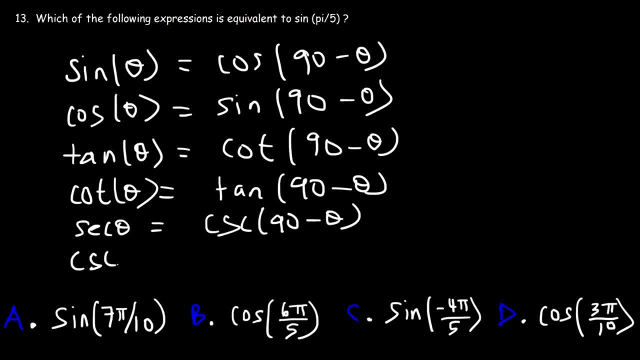 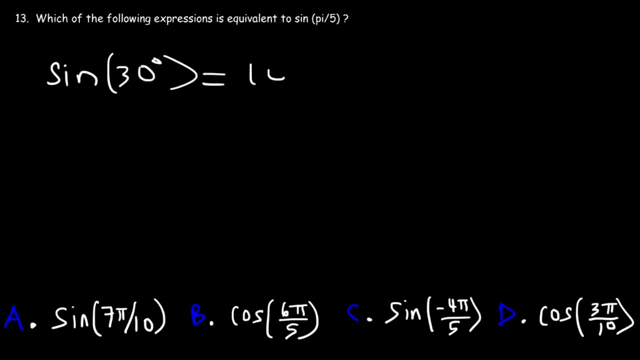 90 minus theta, And for cosecant theta it's secant 90 minus theta. So let's go over some examples of this. So, for instance, sine of 30 degrees is equal to cosine 90 minus 30 degrees, which is basically cosine of 60 degrees, Tangent of 40 degrees. 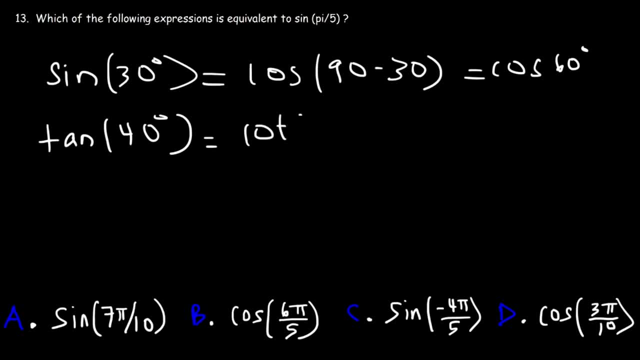 is equal to the co-function of cotangent 90 minus 40 degrees, And so 90 minus 40 is 50.. to cotangent of 50 degrees, Secant of 20 degrees is equal to cosecant of 90 minus 20 degrees. 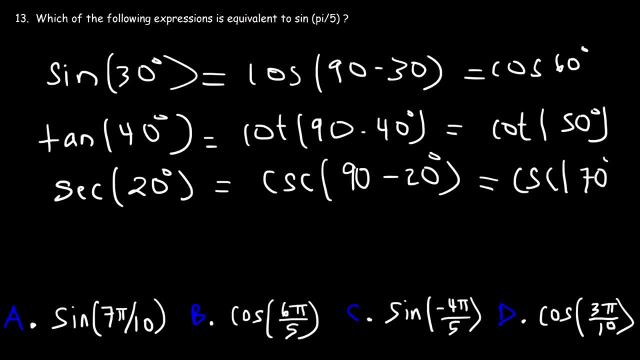 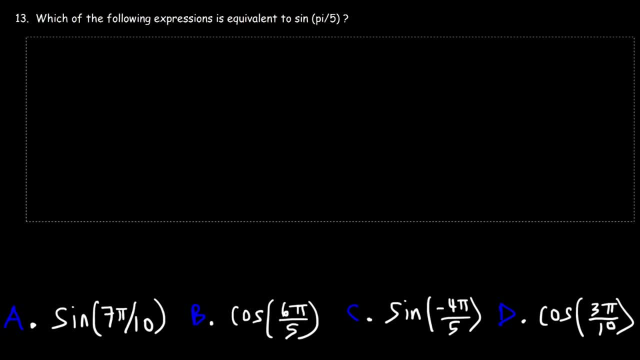 So 90 minus 20 is 70. So that's a quick and simple way in which you can identify the equivalent co-function expression. So now we have our angle in radians, not in degrees, And 90 is equivalent to pi over 2.. Keep in mind that pi is equal to 180.. Half of pi is pi over 2 and half of 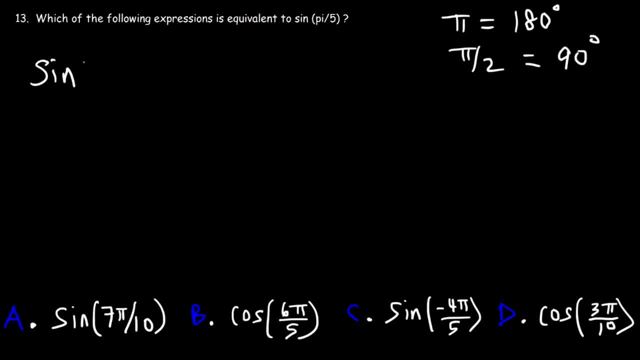 180 is 90. So 90 is the same as pi over 2.. So sine pi over 5 has to be equal to cosine 90 minus pi over 5, or pi over 2 minus pi over 5.. So we need to subtract these two angles. 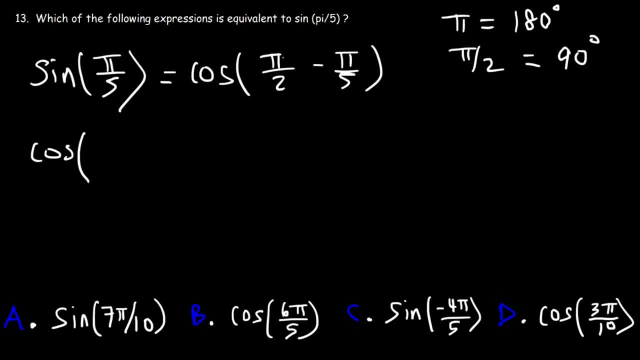 So we need to get common denominators. So I'm going to multiply pi over 2 by 5 over 5.. And pi over 5, I'm going to multiply that by 2 over 2.. So 5 times 2 is 10.. So this is: 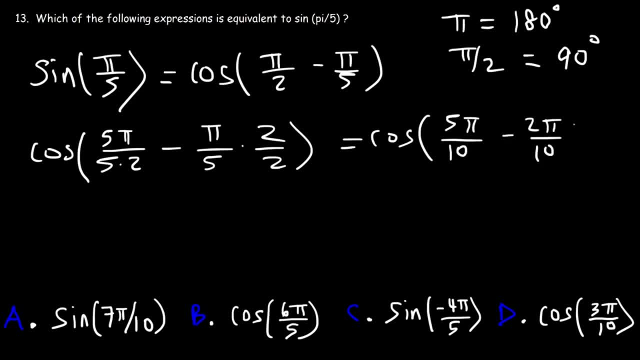 going to be 5 pi over 10 minus 2 pi over 10.. And 5 minus 2 is 3.. So this is equal to 3 pi over 10.. So this is the answer. It's cosine 3 pi over 10,, which means D, is the right answer. Now, if you have, 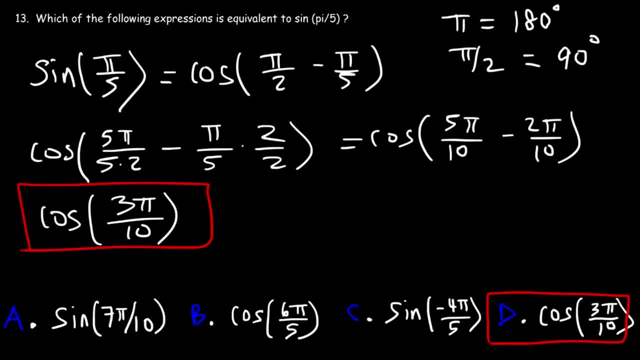 a calculator, you can simply plug everything in, But make sure your calculator is in radian mode, not in degree mode. So if we type in sine pi over 5, this is equal to 0.588.. So that's the answer. 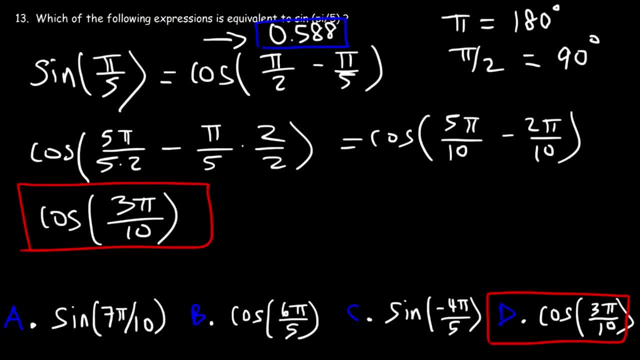 that we need to get. So let's start with answer choice A. Let's type in sine 7 pi divided by 10.. So this is equal to positive 0.809.. Now let's move on to B: Cosine 6 pi divided by 5.. So this is equal to negative 0.809.. 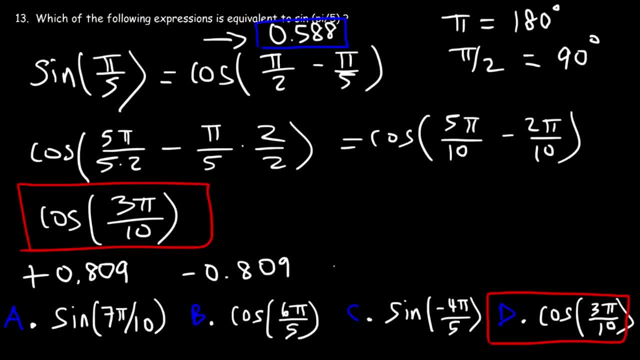 And then part C, sine negative 4 pi divided by 5. This is negative 0.588.. It's close, but it's not the answer. Now for D, cosine 3 pi over 10. This is positive 0.588.. So this is the answer we're looking for. Therefore, D is the right. 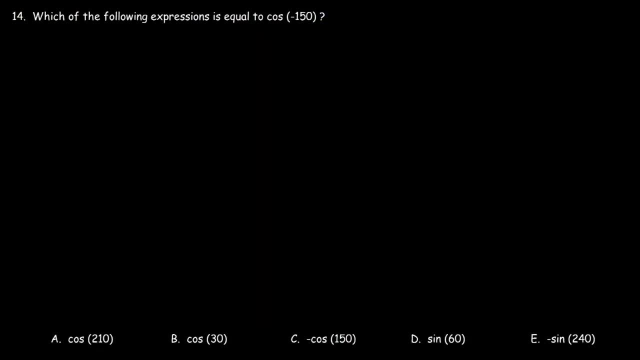 answer: choice Number 14.. Which of the following expressions is equal to cosine negative 150?? So now let's talk about how we can do this without using a calculator or a unit circle or a special reference triangle. So what do you think we can do? 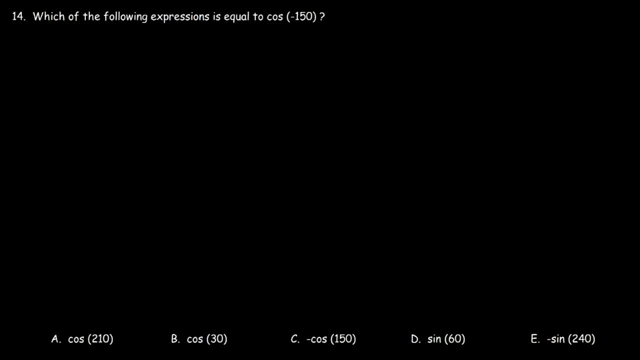 Well, for one thing, we can start with the co-function identity, because we do have some values in sine. So we know that cosine theta is equal to sine 90 minus theta, So we have cosine of negative 150.. So therefore, this is equal to sine 90 minus. 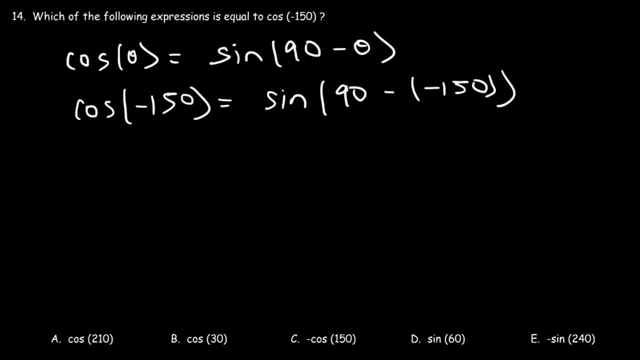 theta, which is negative 150.. So 90 minus negative 150.. That's the same as 90 plus 150, so that's sine 240.. Now E would be correct if there wasn't a negative sine, so therefore we could eliminate answer. 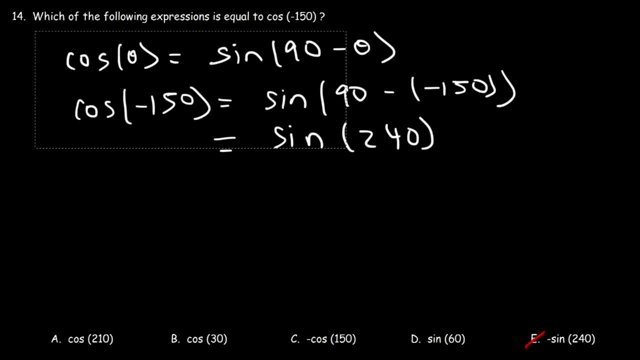 choice E. Now what else can we eliminate? Now let's check out the even-odd properties of cosine. So cosine is an even function. We know that cosine negative x is just cosine x. So what this means is that cosine negative 150 is equal to cosine positive 150. 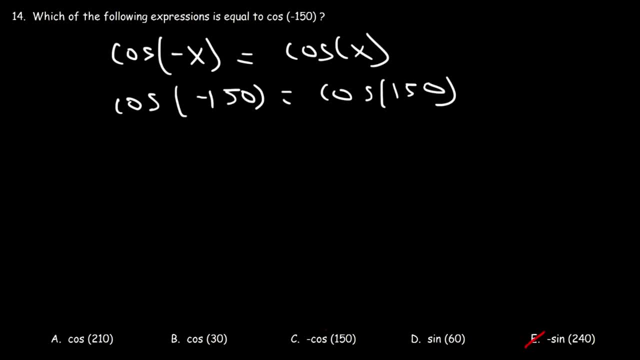 Now, C is close to that, but there's a negative sign in front of it, so we could eliminate answer choice C. Now what about the rest, A, B and D? What can we do? The next thing we could do is look at the sine of cosine. 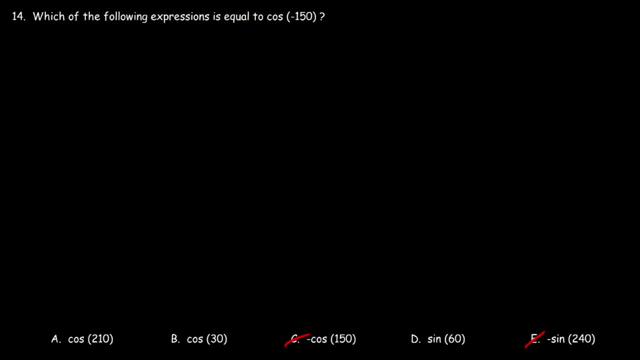 Is it positive or is it negative, depending on certain quadrants. So A is negative. Let's make two graphs. So if we have a positive angle, this is 0,, 90,, 180, and 270.. And if we're dealing with negative angles, this is 0, negative, 90, negative, 180, negative. 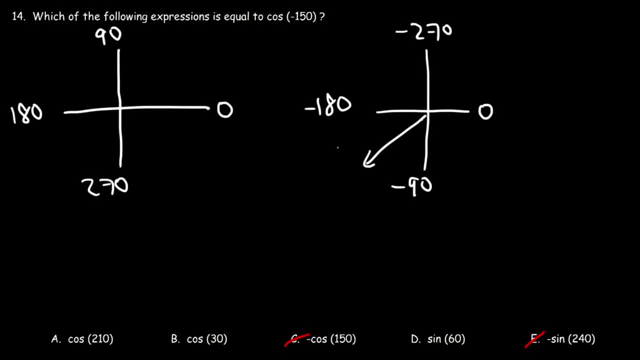 270.. So negative 150 is located in quadrant 3.. So that's for this angle And cosine is negative in quadrant 3 because x is negative in quadrant 3.. So we're dealing with the left side. So we need a negative value for cosine. 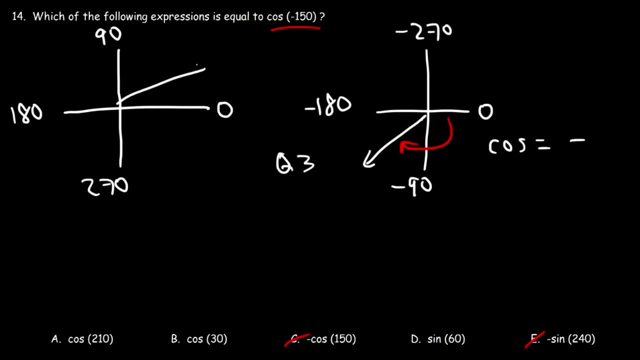 Now looking at answer choice B, 30 is over here, That's in quadrant 1.. So cosine 30 is equal to a positive value, which means we can eliminate answer choice B. And then if we look at sine 60,, 60 is also in quadrant 1, and both sine and cosine are. 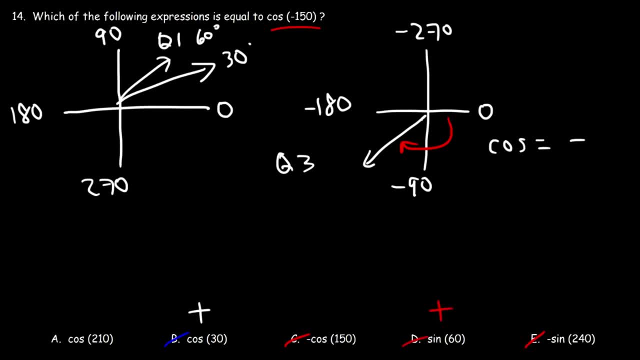 positive in quadrant 1.. So we can eliminate answer choice D. Now 210 is in quadrant 3. And so cosine is negative in quadrant 3.. So A has to be the answer. Another way in which you can confirm that A is the answer is using the periodic properties. 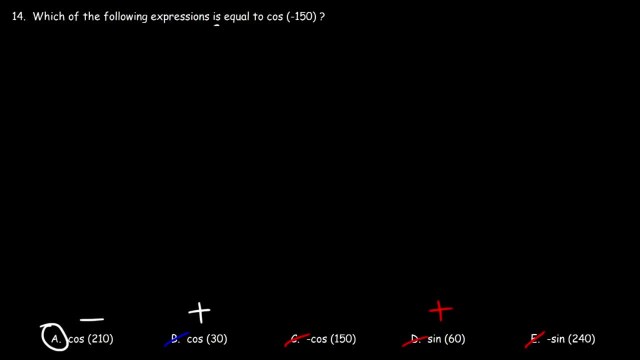 of trigonometric functions. So, for instance, sine of 60 is equal to the sine of a coterminant angle Such as 60.. 60 plus 360,, which is 420.. Or if you do 60 minus 360,, which is negative 300. 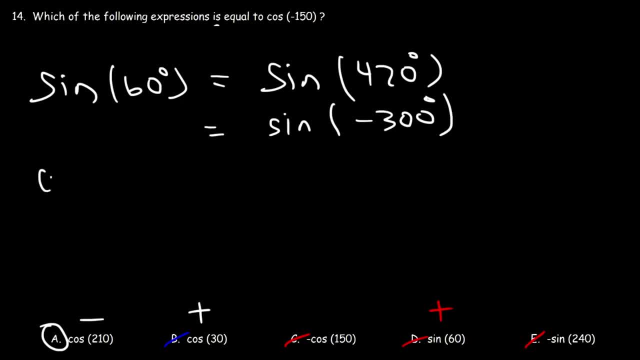 So these are periodic properties of the trigonometric functions. So cosine of an angle is equal to cosine of that same angle plus or minus 2pi or 360 degrees. So we have cosine of negative 150.. That's going to be equal to cosine of negative 150 plus 360.. 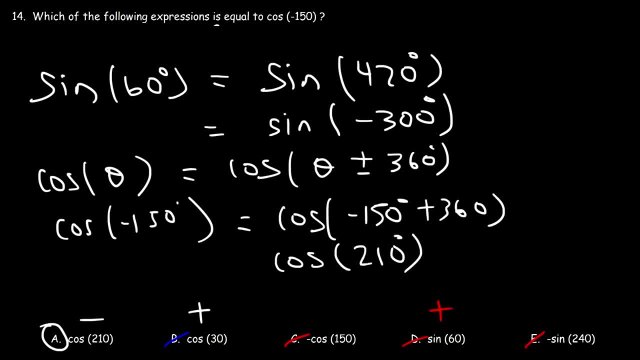 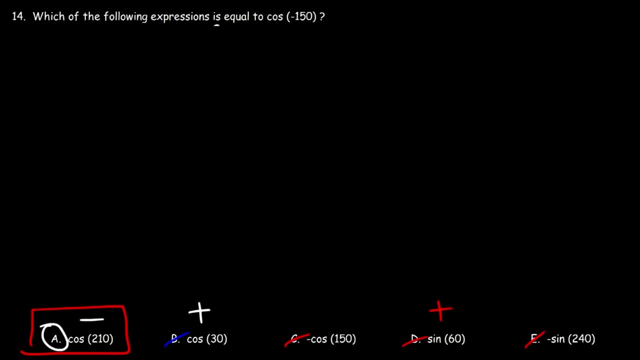 And so negative 150 plus 360,, that's 210. And so that shows that A is indeed the correct answer. Now, for those of you who might be taking a test or a final exam or midterm, and if your teacher allows you to use a calculator, 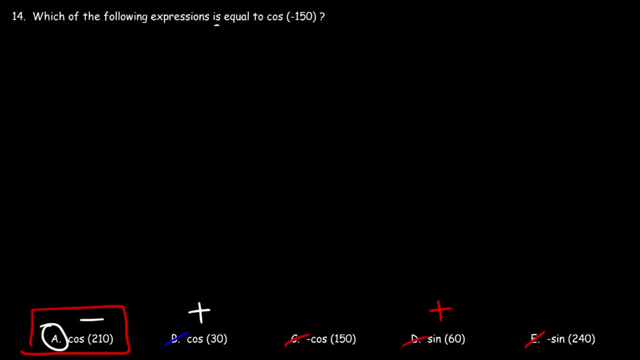 I would highly recommend that you use it for a problem like this, Because it'll make the whole problem a lot easier. So first make sure your calculator is in degree mode. If you don't see a pi next to a number, then the angle is in degrees. 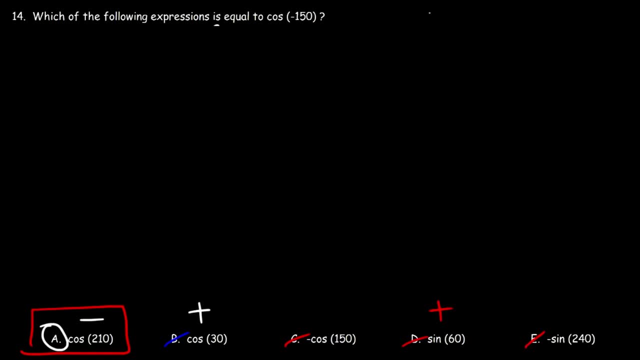 So let's plug in cosine of negative 150.. This is equal to negative square root 3 over 2.. Now if we plug in cosine 210.. We're going to get the same answer, Okay, Okay, So we have the same answer: negative square root 3 over 2.. 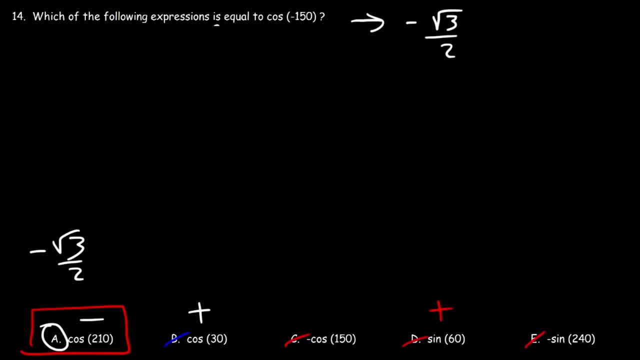 Now my calculator just gives it to me in that form. Your calculator might write it like this: It might display it as negative .866.. And so for answer choice A, it's the same Cosine. 30 is positive square root 3 over 2, but you might see it as positive .866.. 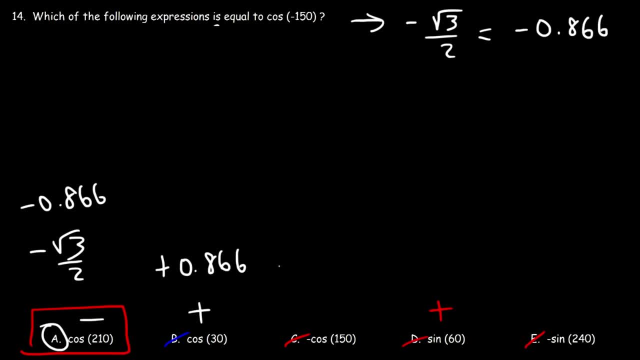 And negative cosine 150.. This is equal to positive .866.. Sine 60 is also positive .866.. And negative sine 240.. That too is positive .866.. So those are all equal to each other. The only one that's different is A, But A is the answer. 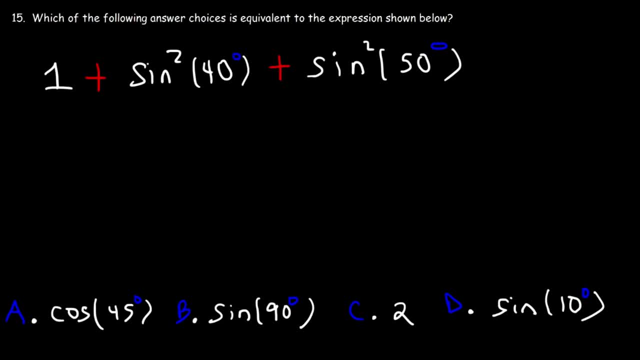 Fifteen, Which of the following answer choices is equivalent to the expression shown below? So, Sine squared of 40 degrees plus sine squared of 50 degrees, Is that equal to cosine 45, sine 90, 2, or sine 10?? 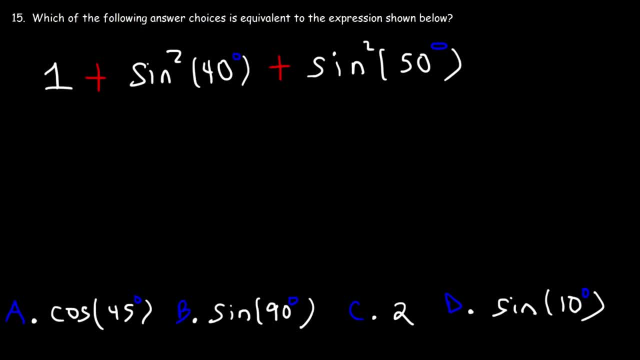 So how can we find the answer to this problem? And what if we don't have access to a calculator? Because if we have access to a calculator you could just type in the whole thing, get the decimal value and then type in each answer choice and see which one matches the answer. 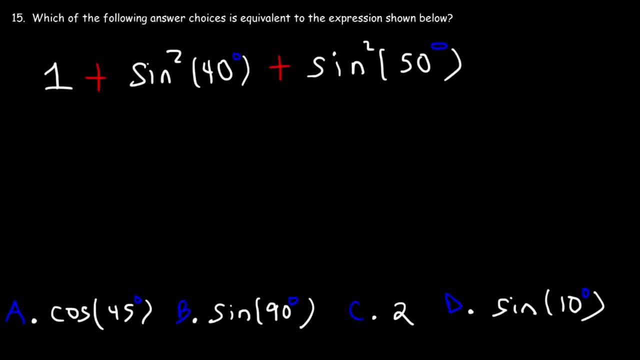 above, So That technique can also be used to find the answer. So Okay, So this can always work for these types of problems if you have access to a calculator. But now let's assume that we don't have access to a calculator. 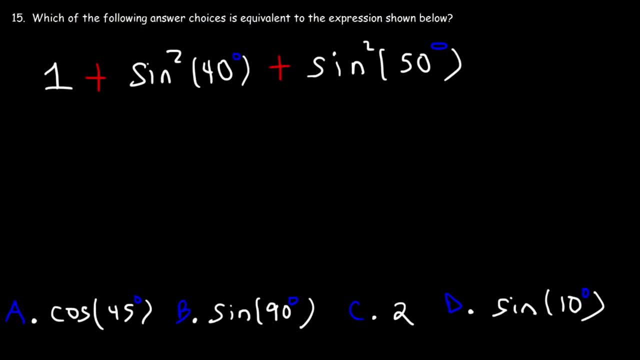 What should we do? Well, for one thing, we can use the co-function properties of sine. So recall that sine theta is equal to cosine 90 minus theta. So sine 50 is equal to cosine 90 minus 50.. And 90 minus 50 is 40.. 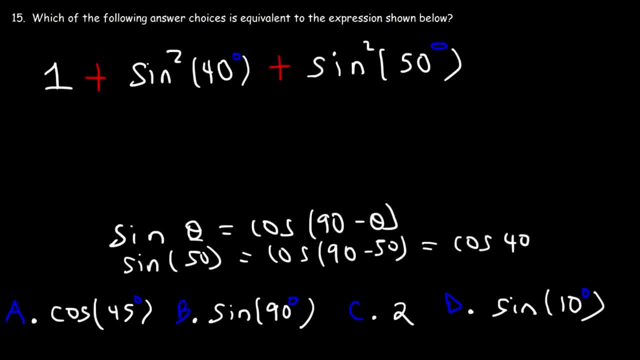 If we square both sides, we can say that sine squared of 50 is equal to cosine squared of 40. Therefore, let's replace sine squared of 50 with cosine squared 40.. Now we can use another identity, and that is the pythagorean identity for cosine and. 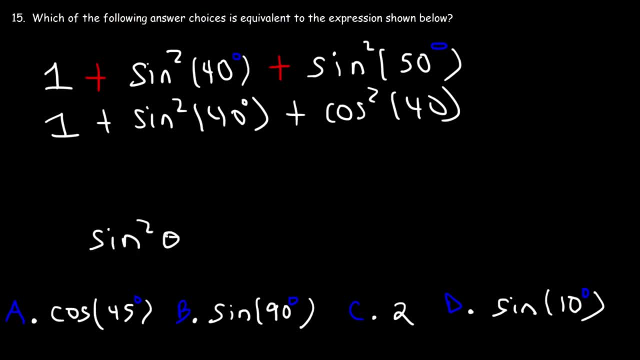 sine. So sine squared plus cosine squared is equal to 1 if the angle is the same, which in this case it is. So we can replace this part sine squared plus cosine squared of 1.. So the answer becomes 1 plus 1, which is equal to 2.. 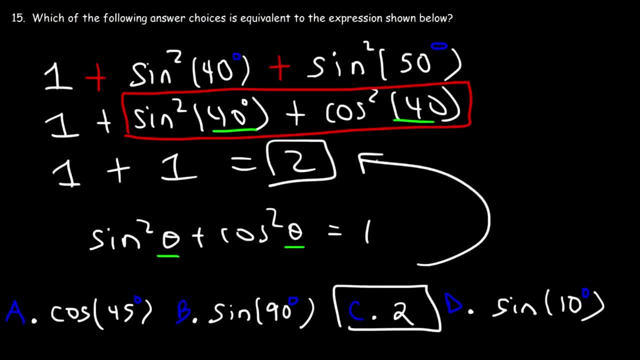 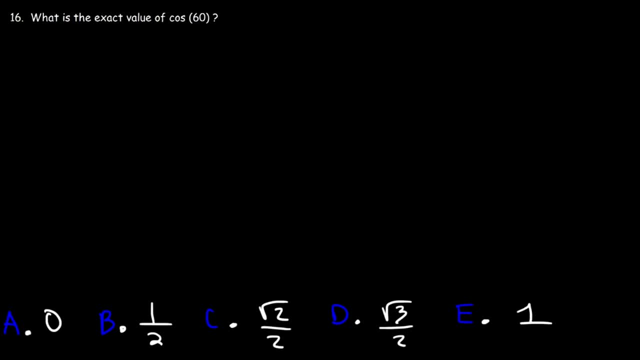 So therefore, C is the right answer in this problem, Number 16.. What is the exact value of cosine 60?? Don't use a calculator, That's just going to be too easy. So there's two other ways to find the answer if you don't have access to a calculator. 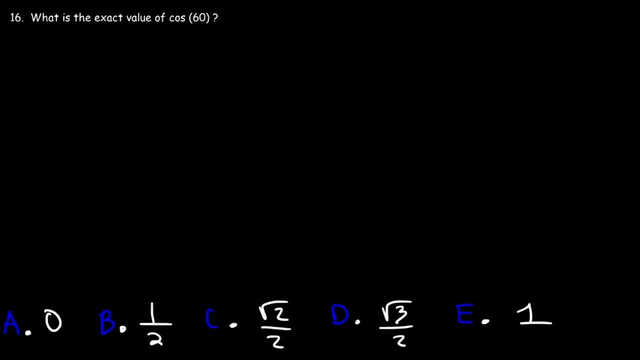 You can use a 30-60-90 reference triangle or you could use a unit circle, But let's focus on a reference triangle first. So let's say this is 30 and this is 60. Across the 30,, the side value is 1.. 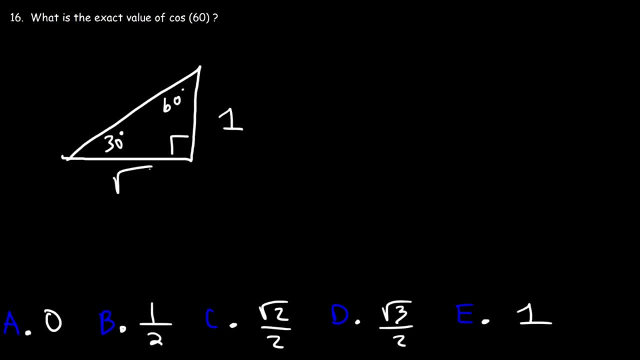 Across the 60, the side length is equal to the square root. Across the 90, the hypotenuse is 2.. So if you memorize this triangle, it can help you to find the value of sine 30 or cosine 60 and things like that. 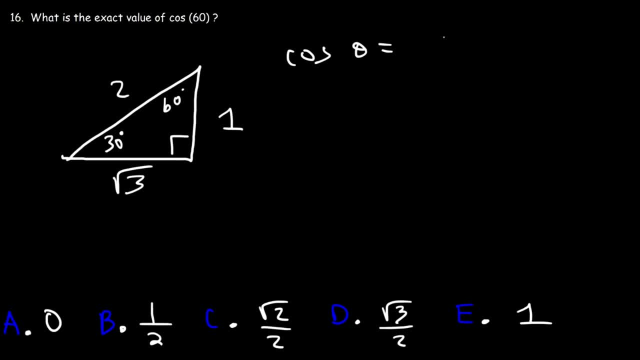 So recall that cosine theta is equal to the adjacent side divided by the hypotenuse based on SOHCAHTOA. So we want to evaluate cosine of 60. So we need to focus on the 60 degree angle. Now, 2 is clearly the hypotenuse. 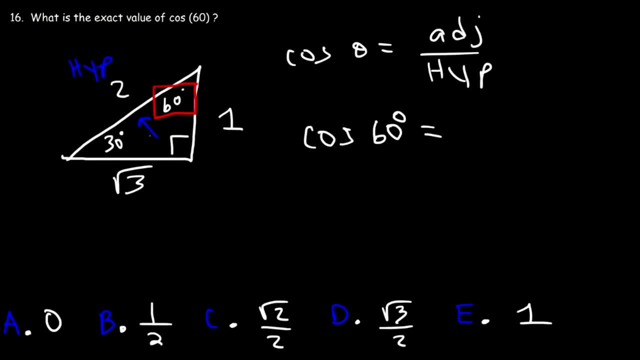 That's always going to be the case. Opposite to 60 is the square root of 3.. So 1 must be the adjacent side, So it's adjacent over hypotenuse. That means it's 1 divided by 2.. 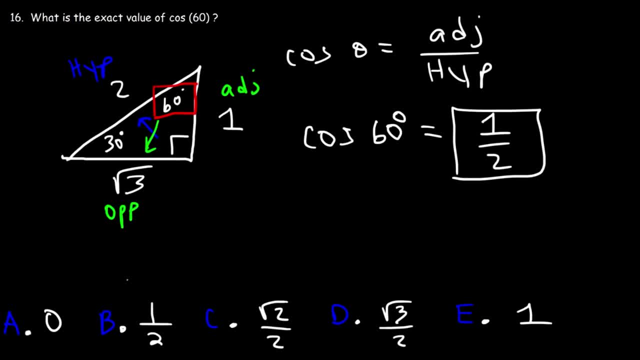 And so that's how you can find the exact value of cosine 60,, which means that answer choice B is the correct answer. Now let's say if you have access to the unit circle or if you want to commit the unit circle to memory. 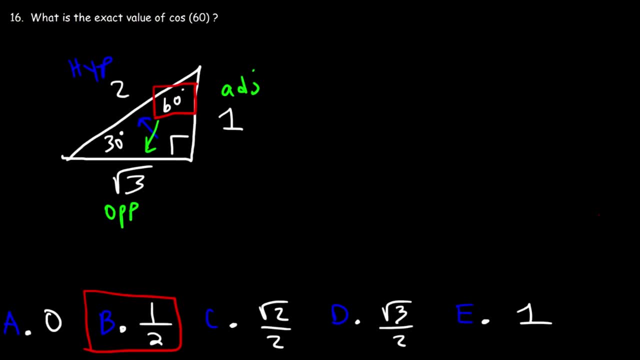 By the way, if you need a copy of the unit circle, go to Google Images And type in unit circle and you should see a bunch of it pop up. Now in the unit circle, at an angle of 60 degrees or pi over 3, you'll see these values. 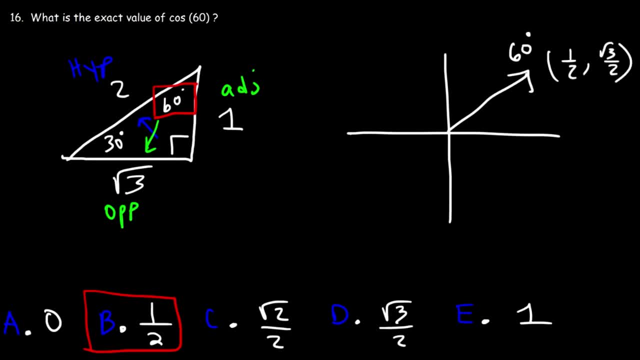 1 half comma, square root 3 over 2.. Now for a unit circle. keep in mind that sine theta is equal to y and cosine theta is equal to x. Well, in this example, theta is 60. So cosine 60 is equal to the x value, which is 1 half. 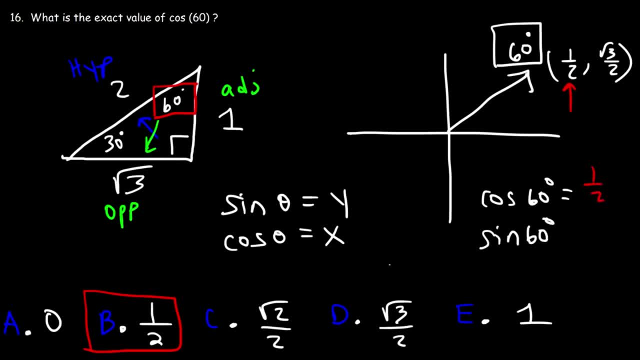 And sine 60,, for example, is equal to the y value, which is the square root of 3 over 2.. So that's how you can use the unit circle to evaluate certain trigonometric functions with their angles. So in this case, B is the right answer. 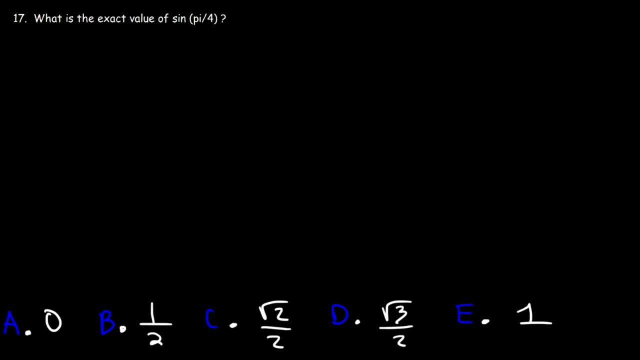 Number 17,. what is the exact value of sine pi over 4?? First, let's convert the angle from radians to degrees, So it's pi over 4, and we're going to multiply it by 180, divided by pi. 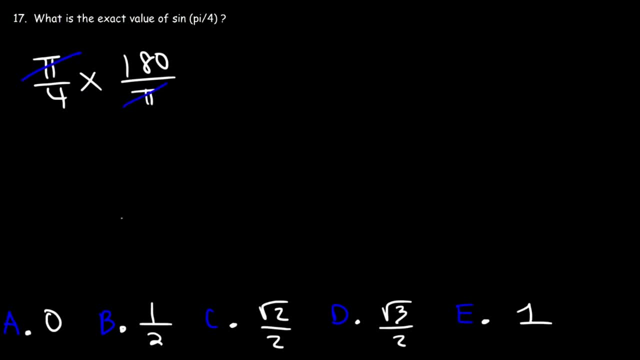 So basically, we're replacing pi with 180. And so we're going to get 180 over 4, because pi equals 180.. So what's 180 divided by 4?? So how can we find the answer for that? 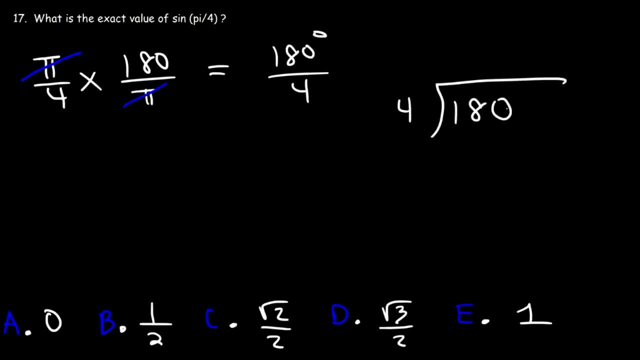 Well, if you don't have access to a calculator, you could use long division. 4 goes into 18. four times 4 times 4 is 16. And 18 minus 2 is I mean 18 minus 16 is 2.. 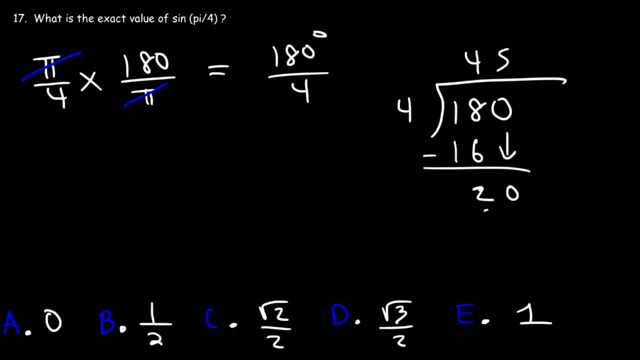 And then bring down to 0.. 4 goes into 25 times, And so the remainder is 0. So 180 divided by 4 is 45. So we need to find the value of sine 45 degrees. 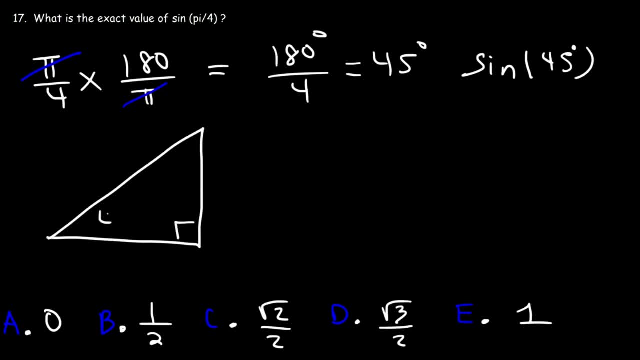 So we need to use the 45-45-90 reference triangle. So this is another one that you want to commit to memory Across the 45 degree angles. it's 1.. The hypotenuse is the square root of 2.. 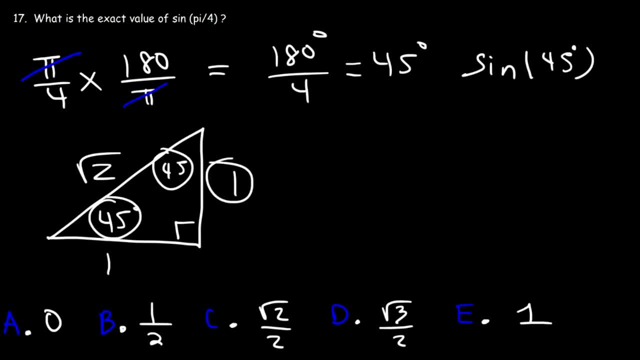 Because the angles are the same, the side lengths have to be the same. So now recall that sine is equal to opposite divided by hypotenuse. So let's pick one of the angles Opposite to 45 is 1.. 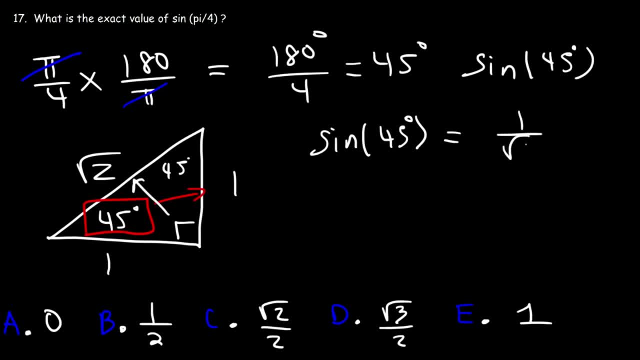 And the hypotenuse is 1.. So we need to use the square root of 2.. Now we need to rationalize the denominator, So we're going to multiply the top and the bottom by the square root of 2.. 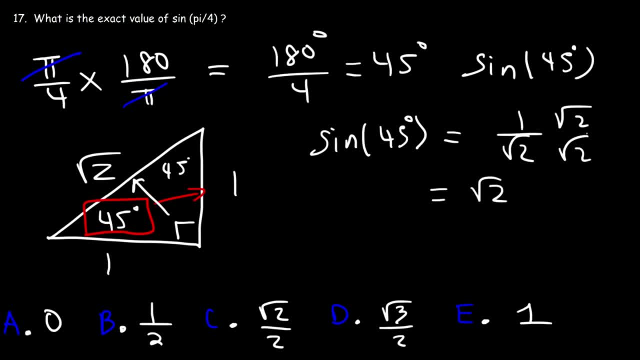 So 1 times the square root of 2 is the square root of 2.. The square root of 2 times the square root of 2.. We know that 2 times 2 is 4.. So that becomes the square root of 4, which is equal to 2.. 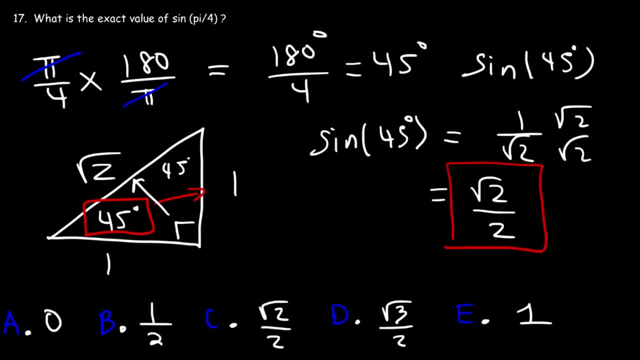 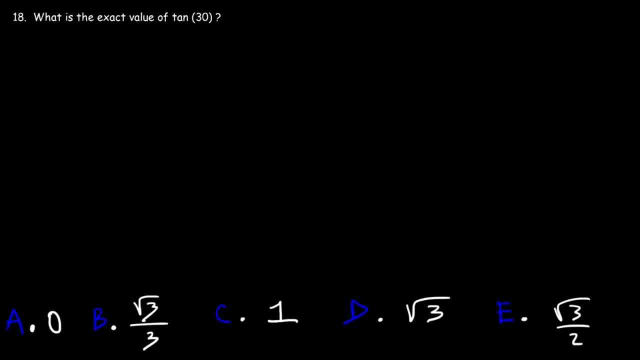 So sine 45 is equal to the square root of 2 divided by 2.. Which means C is the correct answer 18,. what is the exact value of tangent 30?? So go ahead and try that problem. So let's use the 30-60-90 triangle. 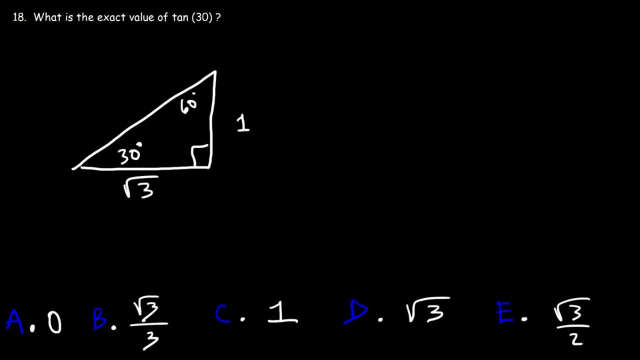 So across the 30 is 1.. Across the 60 is the square root of 3.. Across the 90 is 2.. So recall that tangent of theta is equal to the opposite side divided by the adjacent side, And so we're focusing on the 30-degree angle. 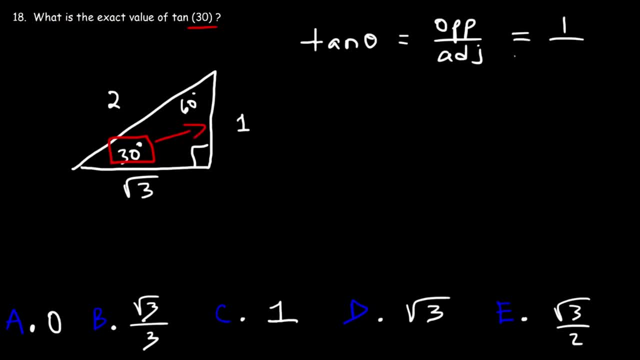 Opposite to 30 is 1.. And adjacent to 30 is the square root of 3.. So we need to rationalize it. So this becomes the square root of 3.. And then the square root of 3 times itself is the square root of 9, which is 3.. 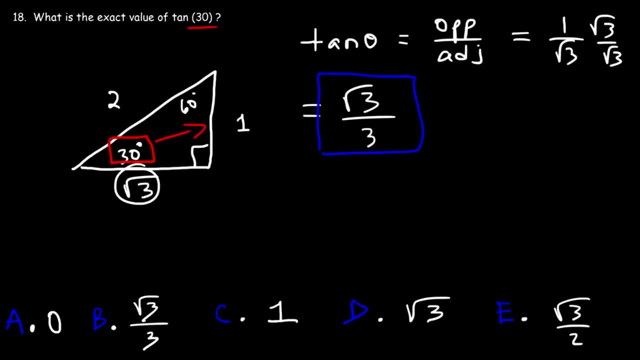 So tangent 30 is root 3 divided by 3.. So B is the right answer. Now, if you wish to use a unit circle to get the answer, here's what you can do. So first you need to locate the 30-degree angle on the unit circle. 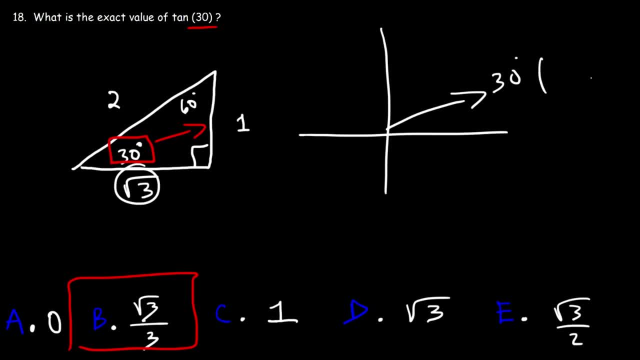 So at 30 degrees you'll see that X is the square root of 3 over 2, and Y is 1 half. Now recall that tangent is sine divided by cosine, It's Y divided by X. So sine, 30 is 1 half. 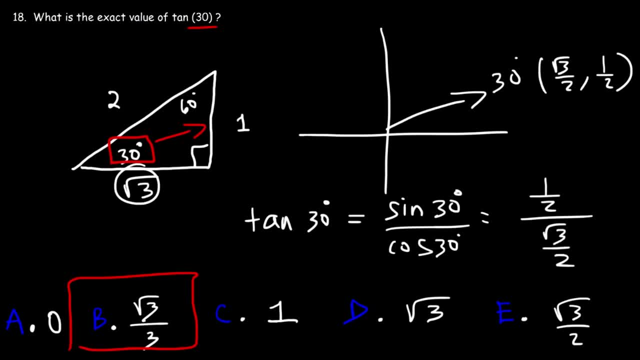 Cosine 30 is the square root of 3 over 2.. Now if we multiply the top and the bottom by 2, we can get rid of some fractions. So on top this is going to be equal to 1.. 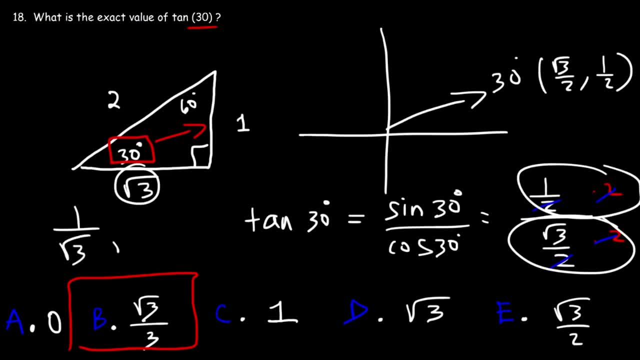 On the bottom, the 2s will cancel and we're going to get the square root of 3.. And then we can rationalize it, giving us the same answer: square root 3 divided by 3.. So B is the right answer. 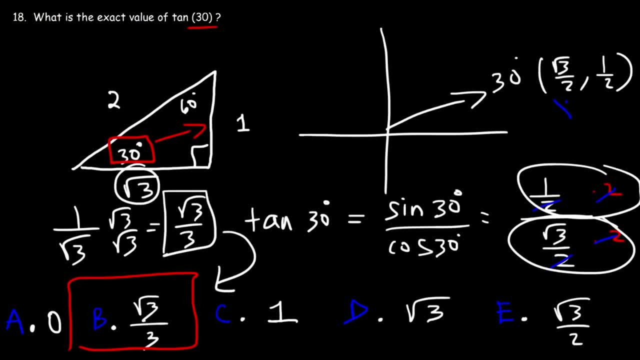 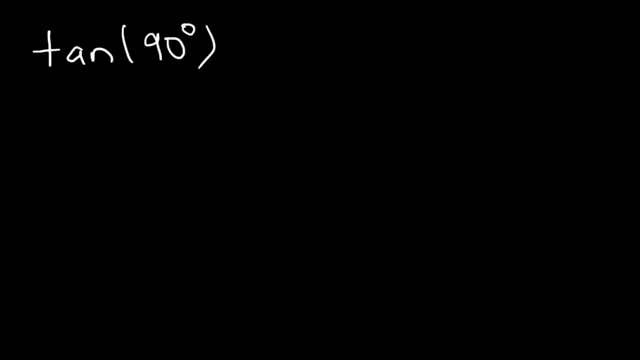 Keep in mind that cosine is associated with the X value And sine is associated with the Y value. Now, as a side question, what is the value of tangent 90?? If you use the unit circle, you need to know that at 90 degrees. 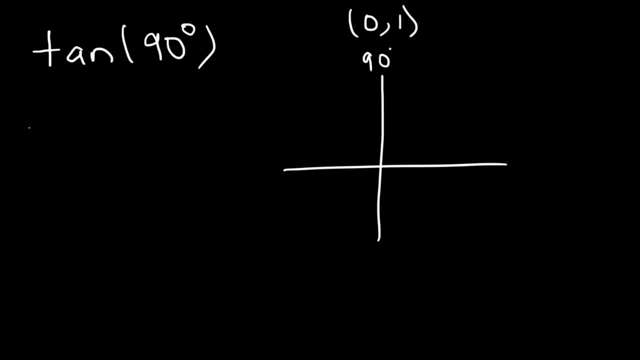 X is 0, Y is 1.. And so tangent 90 is going to be Y divided by X. The Y value is 1, X is 0.. So what's the value of tangent 90? It's 1 divided by 0.. 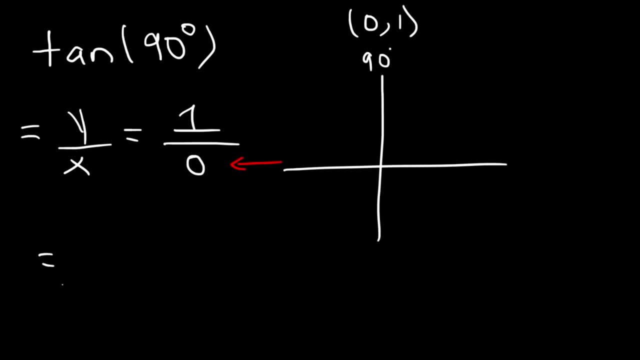 Anytime you get a 0 in a denominator that means that it's undefined. So if you were to type in tangent of 90 in your calculator, make sure it's in degree mode. it's going to give you an error. 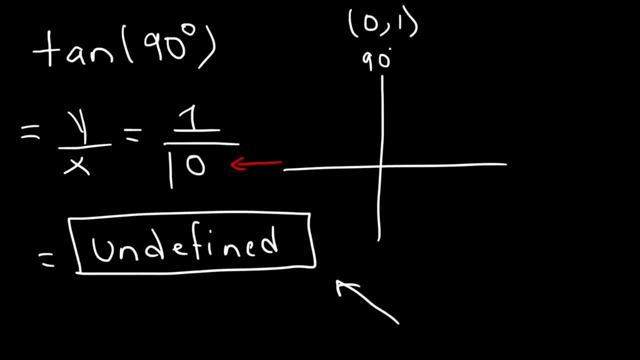 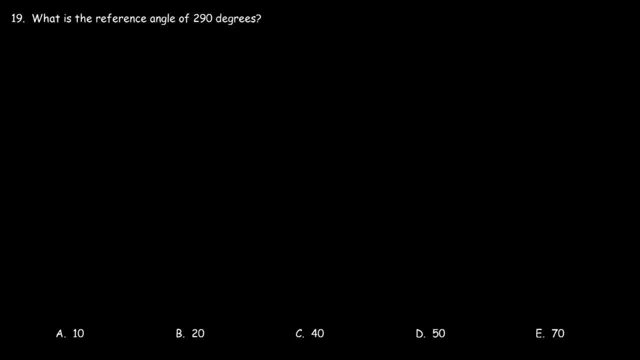 And so when you see that, it means that the answer is undefined, It means that you have a 0 in the denominator of a fraction. So just watch out for that Number 19.. What is the reference angle of 290 degrees? 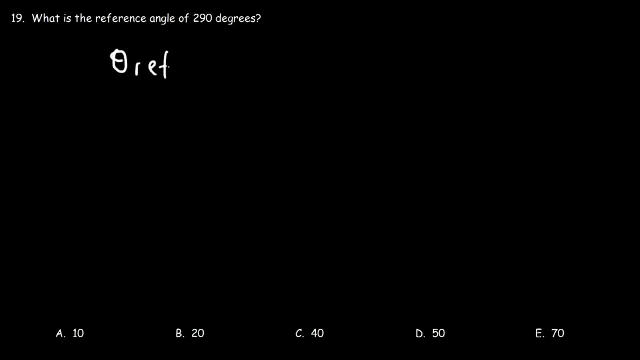 Well, first you need to realize that the reference angle is an acute angle between 0 and 90. So the first thing you need to do is you need to determine what quadrant the angle is in. So let's say, if we have an angle in quadrant 1.. 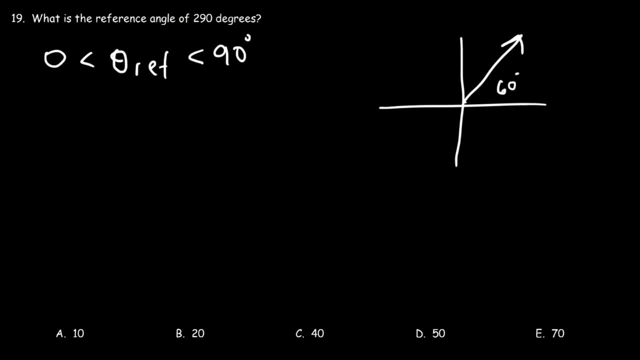 Let's say the angle is 60. The reference angle is the angle between the X-axis and the terminal side of the original angle. So in quadrant 1, the reference angle is equal to or the same as the angle in quadrant 1.. 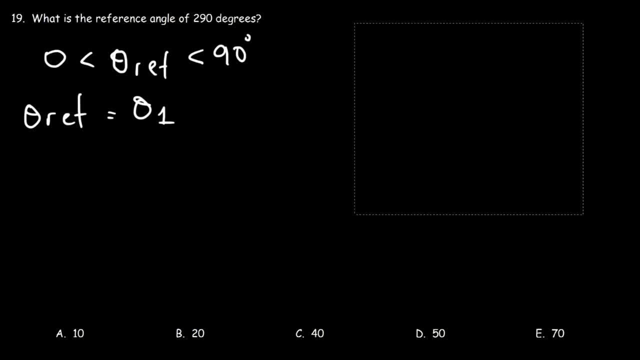 So in this example it is 60 degrees. Now what if we have an angle that's in quadrant 2? Let's say it's 150 degrees. What's the reference angle? So the reference angle is between the X-axis. 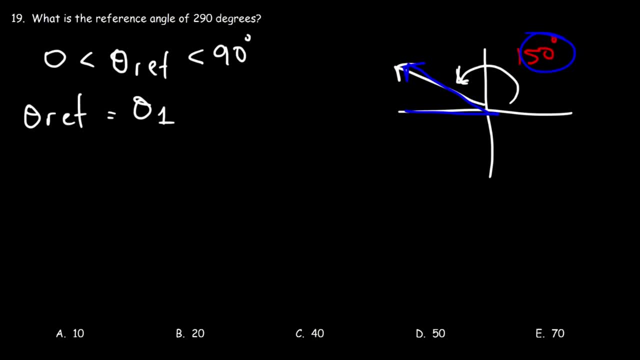 and the terminal side of the original angle. So it's going to be the angle inside here. So going from the positive X-axis to the negative X-axis, that's 180.. Less 150.. So the angle on the inside must be 30.. 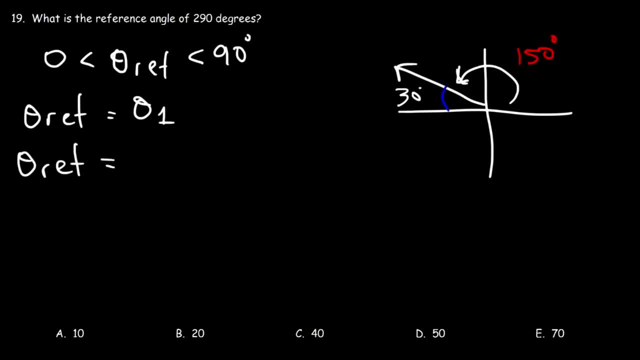 Therefore, to calculate the reference angle for an angle in quadrant 2, it's going to be 180 minus the angle in quadrant 2.. So in this example it was 180 minus 150, which is 30. Now what if the angle is in quadrant 3?? 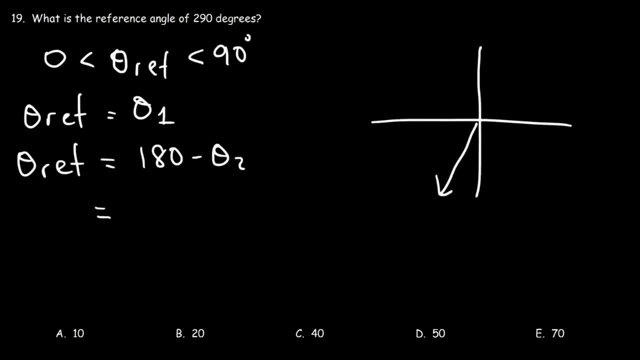 What's the formula? So let's say, if the angle is 240 degrees, How can we calculate the reference angle? So the reference angle is between the X-axis and the terminal side. So that's this angle here, And we know this is 180.. 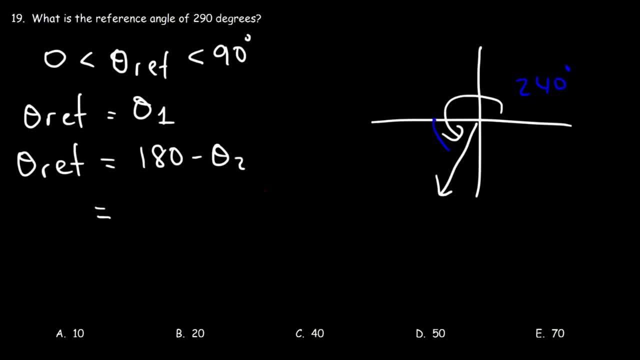 This is 240.. So the difference between those two values is the reference angle, which is 60.. So for an angle in quadrant 3, the reference angle is going to be the angle in quadrant 3 minus 180.. So it was 240 minus 180, and that gave us 60.. 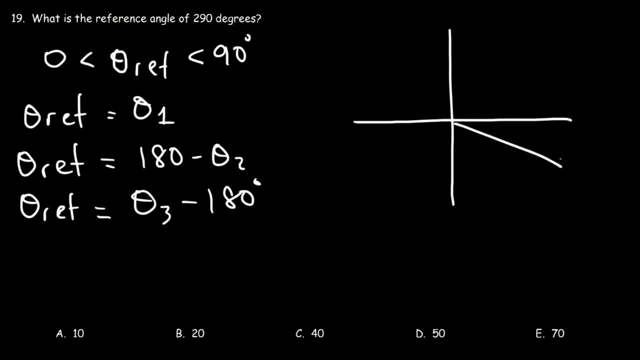 Now let's consider an example in quadrant 4.. So let's use the formula 330 as an example. so we need to find the angle between the x-axis and the terminal side. so that's this angle here. now a full rotation around the circle is: 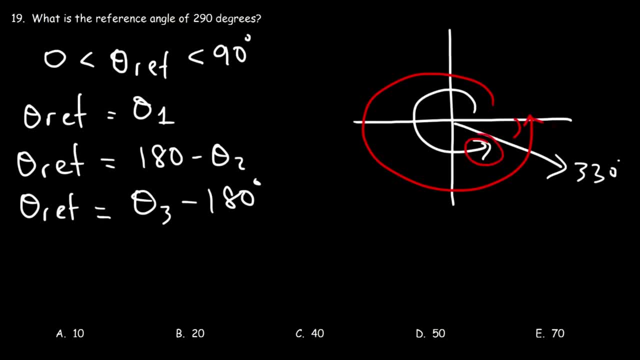 360, so less 330. therefore this angle has to be 30 degrees. so to calculate the reference angle for an angle in quadrant 4, it's always going to be 360 minus the angle in quadrant 4. so those are some formulas that you want to keep in mind. 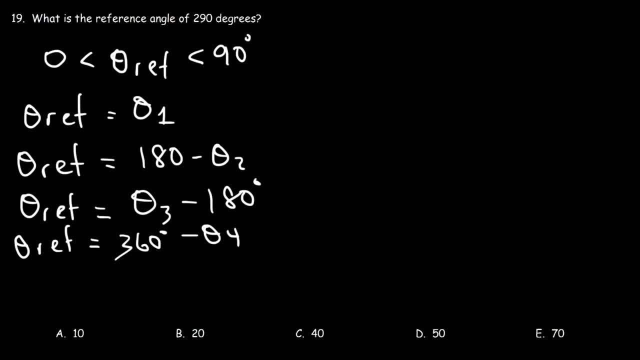 if you wish to calculate the reference angle now, in our example, the angles 290. so the first thing we need to do is identify what quadrant 290 is located in. so this is 0, 90 degrees, 180, 270, and 0 is the same as 360. those two angles are: 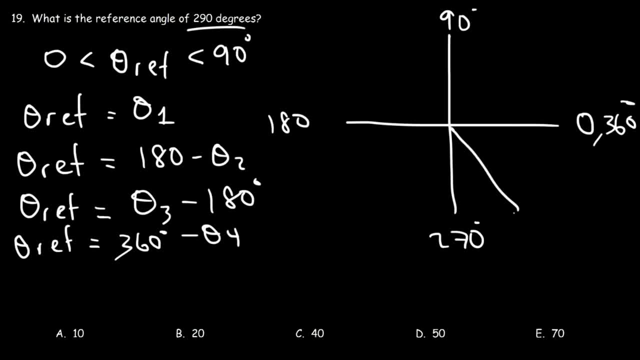 coterminal to each other. so 290 is located in quadrant 4, so therefore need to use this equation. so the reference angle is simply going to be 360 minus the angle in quadrant 4, which is 290. 360 minus 290 is 70, so 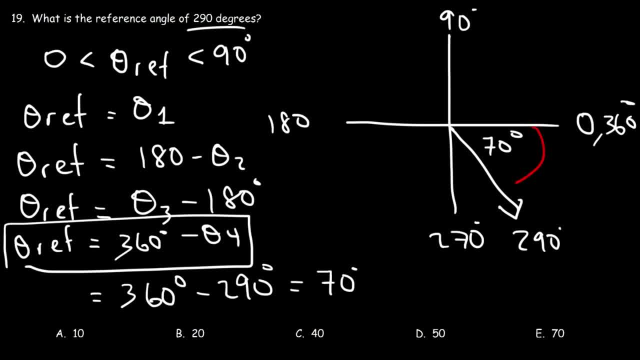 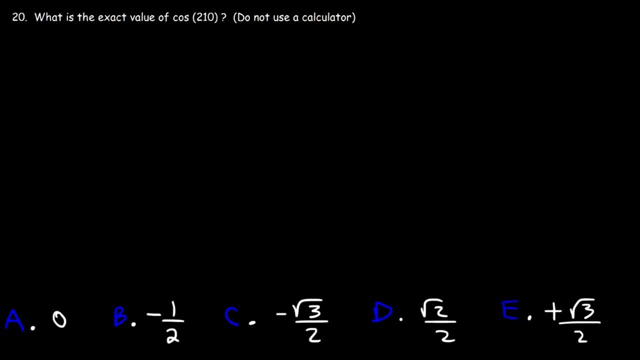 that's the reference angle between the x-axis and the terminal side. it's 70 degrees, which means e is the answer. so now you know how to find a reference angle of any angle, number 20. what is the exact value of cosine 210? and do not use a calculator so we know. this is 090, 180, this is 270, so 210 is located. 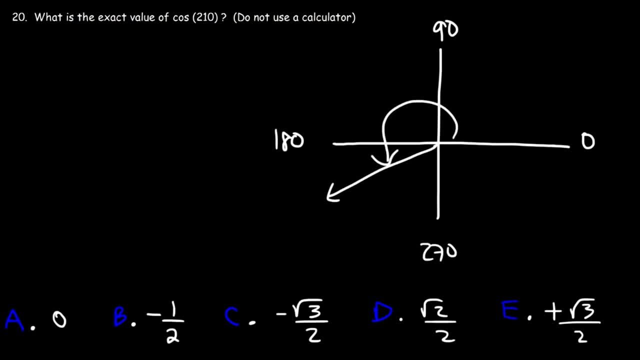 in quadrant 3, so this is an angle of 210. now what we need to do is calculate the reference angle. so for an angle in quadrant 3, the reference angle is the angle in quadrant 3 minus 180, so that's going to be 210 minus 180, and so the 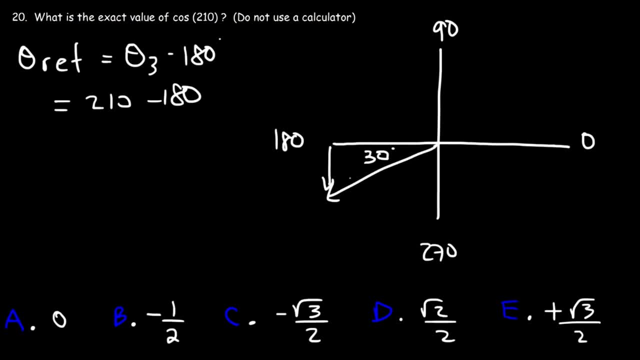 reference angle is 30 degrees, so let's turn this into a triangle now recall the 30- 60, 90 triangle. this is 30, this is 60 across the 30 is 1, across the 60 is root. 3 across the 90 is 2. so now 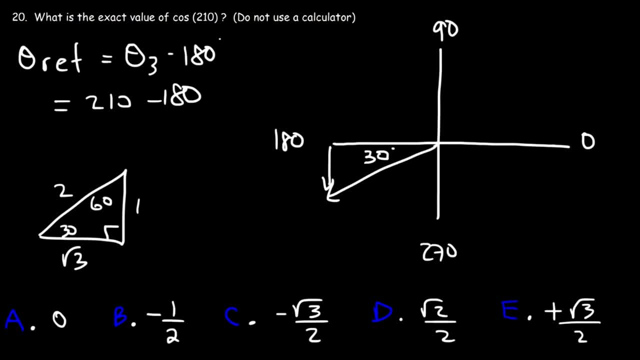 in quadrant 3 across the 30 is also 1, but since we're going along the negative y-axis, this is going to be negative 1. now this is the 90 degree angle, so the hypotenuse has to be 2. so over here is a. 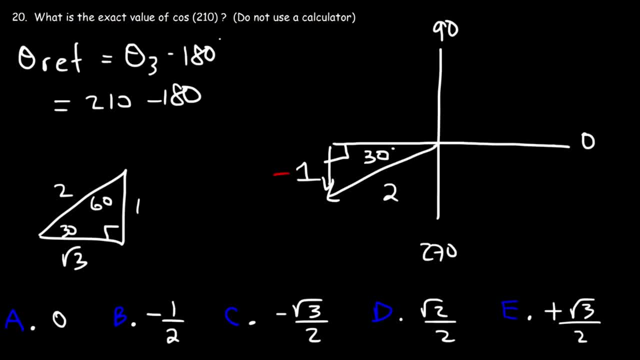 60 degree angle, so across the 60 is the square root of 3. now we're going in the negative x direction, so that has to be negative square root 3. so now we can evaluate cosine of 210 using a 30, 60, 90 reference angle, and that's why it's. 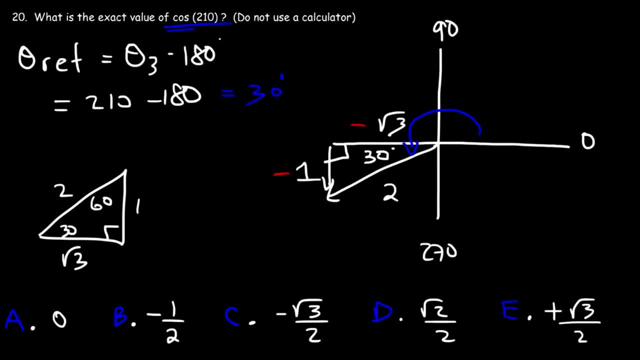 important to calculate the reference angle because it can help you to find the exact value of these functions if you don't have access to a calculator or if you don't have access to a unit circle. so, cosine of 210, which is equal to cosine 30, but cosine 30 is positive, cosine 210 is negative, so it's really.